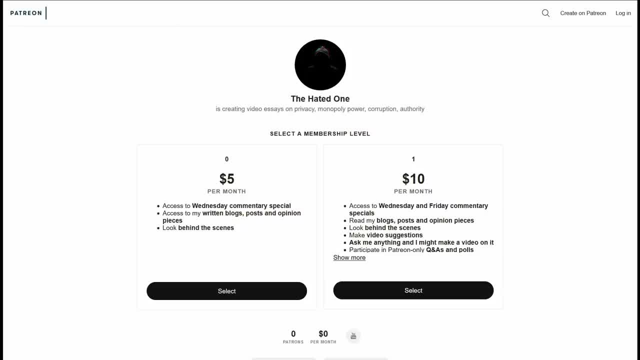 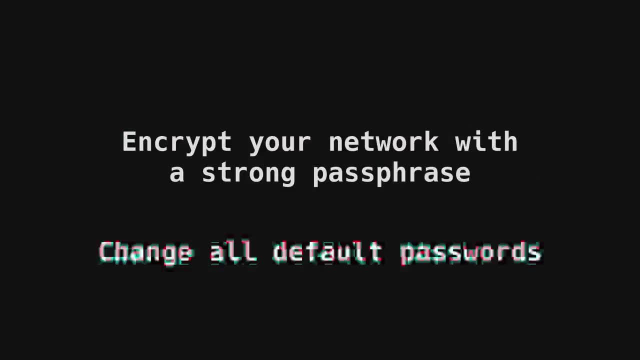 pass on the knowledge to others. If you like this security series, support it on Patreon, because YouTube hates me. The first step you need to make is to make sure your home network is encrypted and all default passwords are changed. This is a very easy step and the most 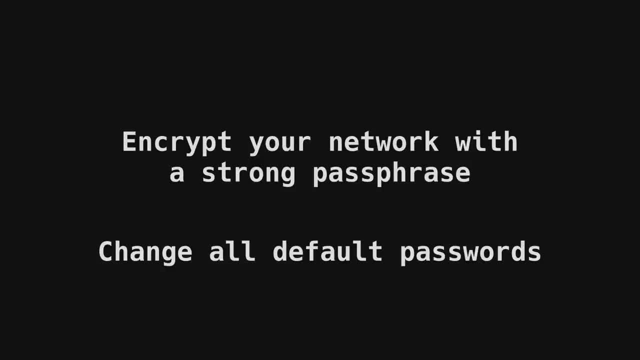 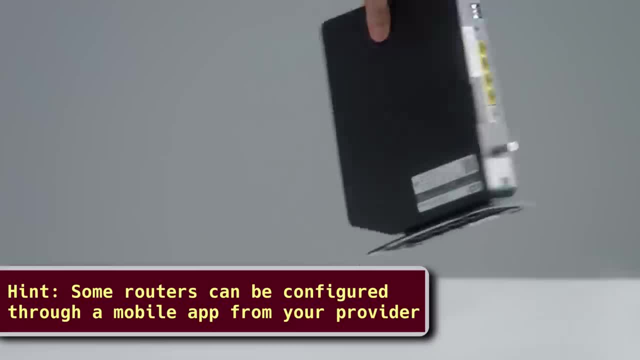 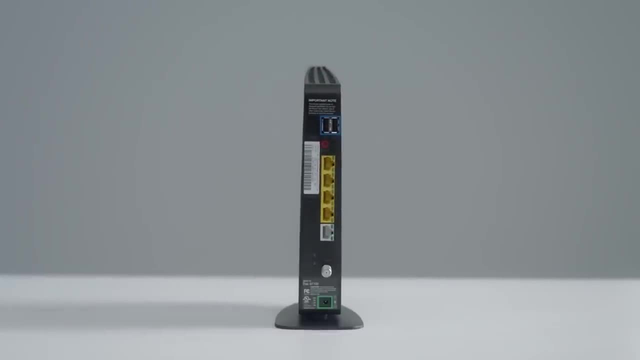 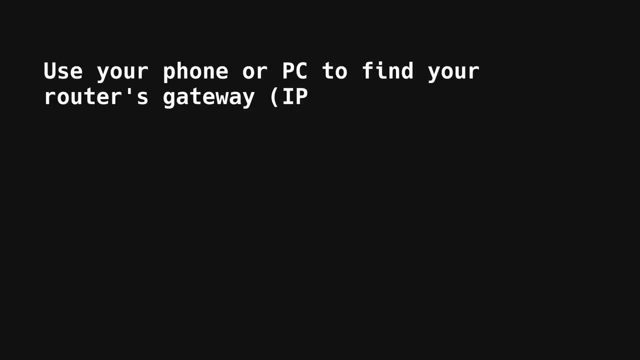 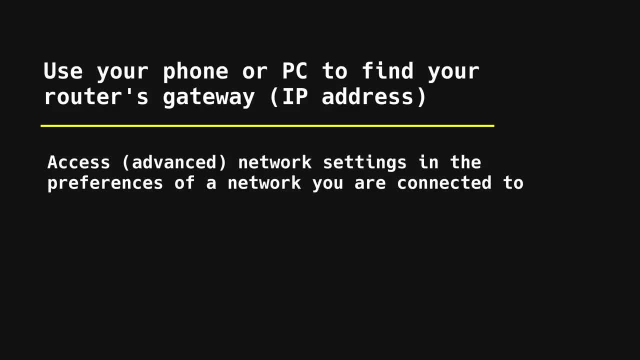 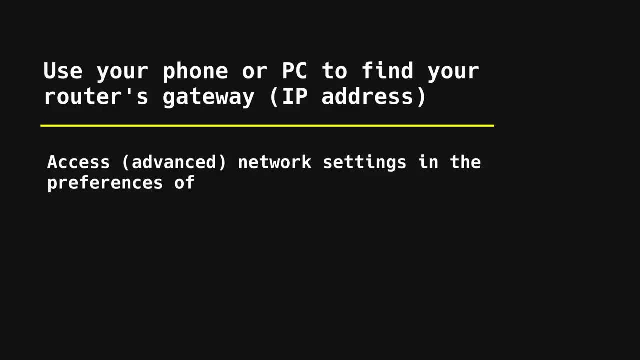 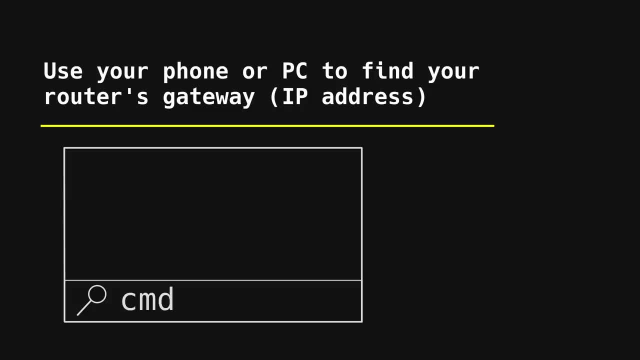 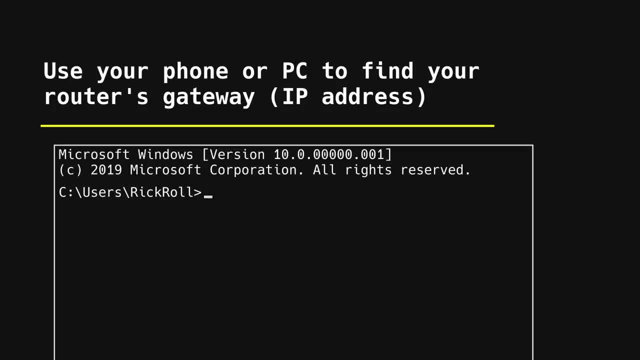 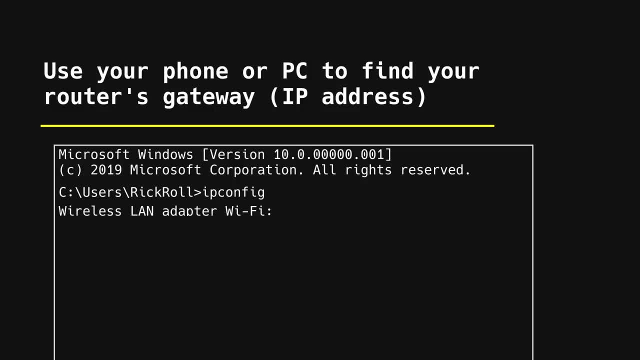 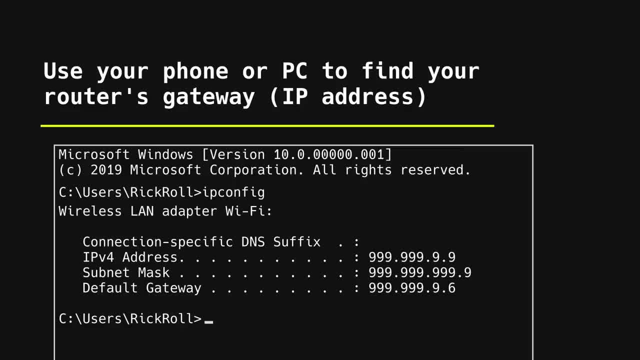 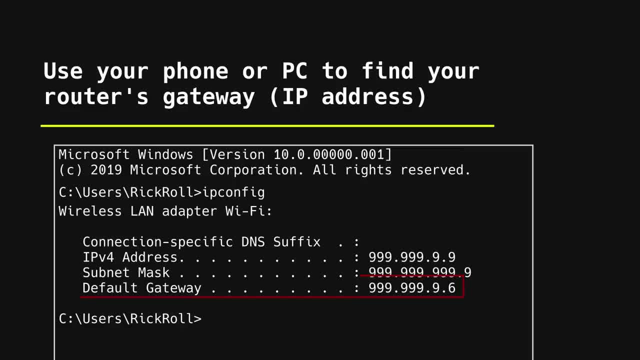 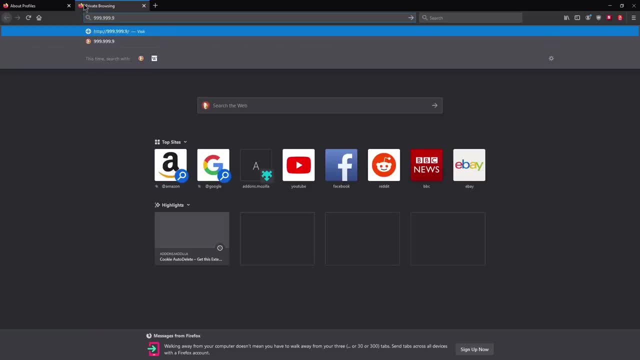 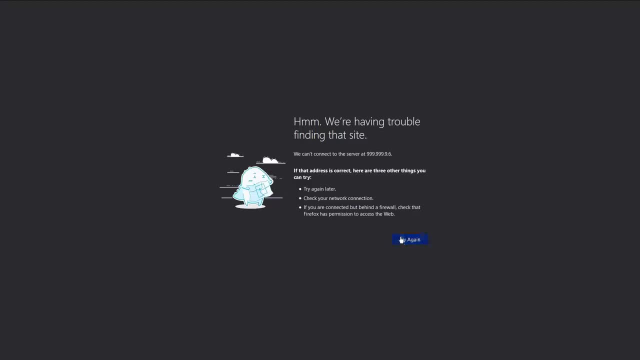 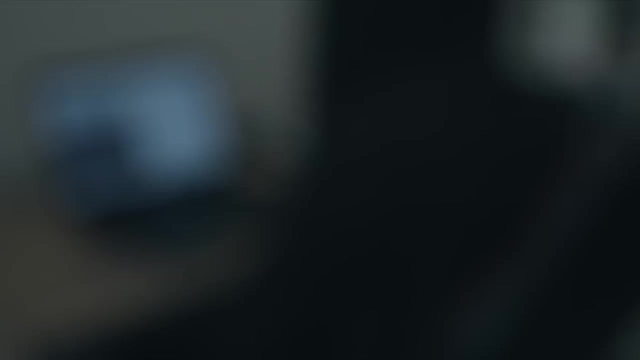 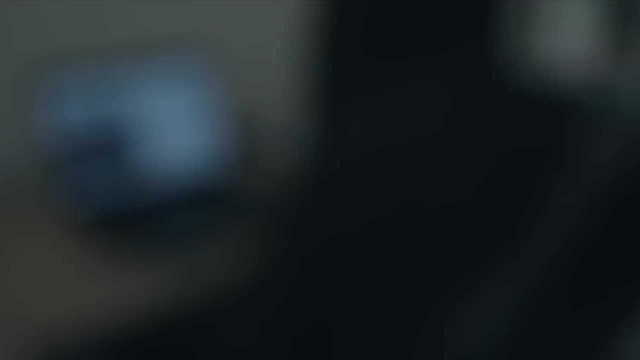 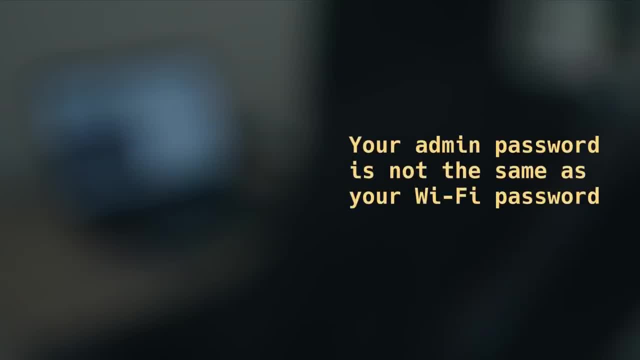 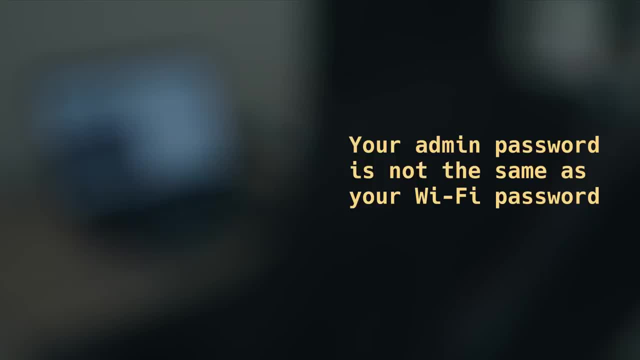 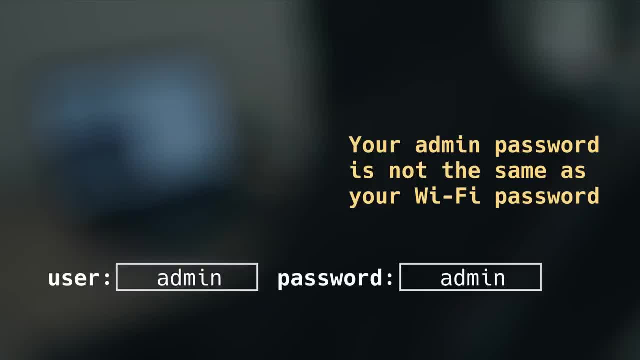 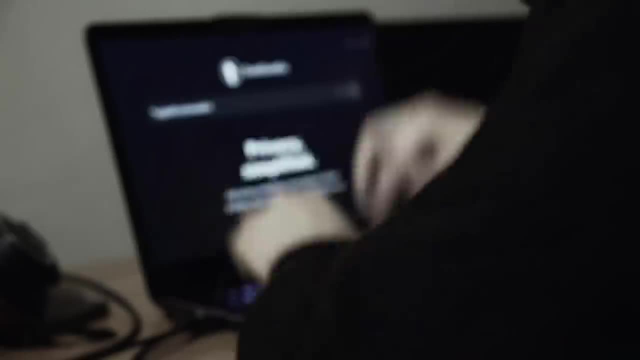 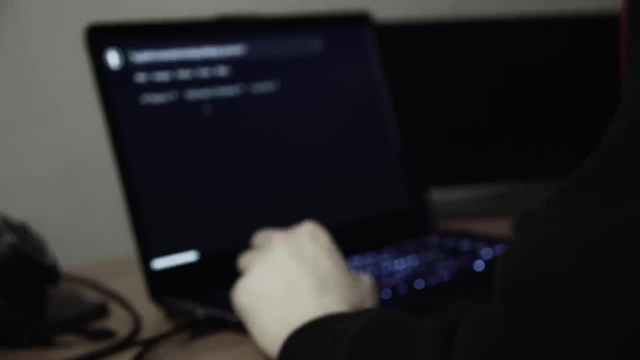 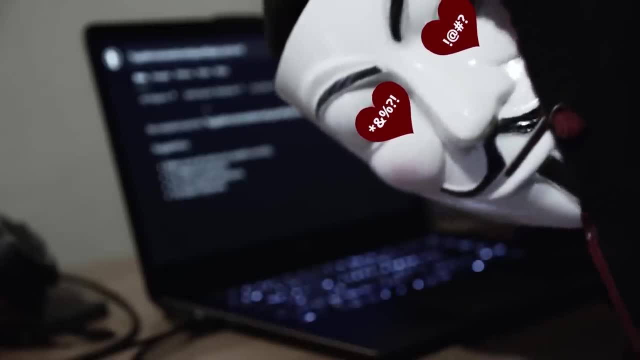 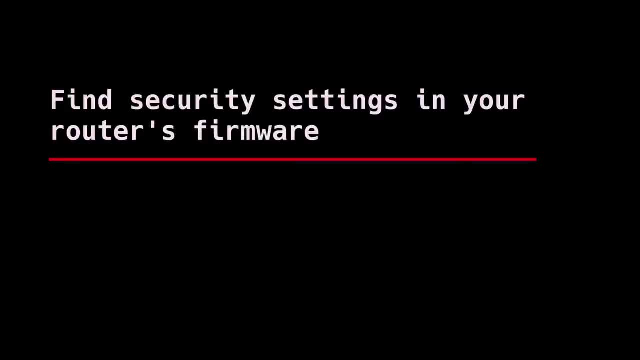 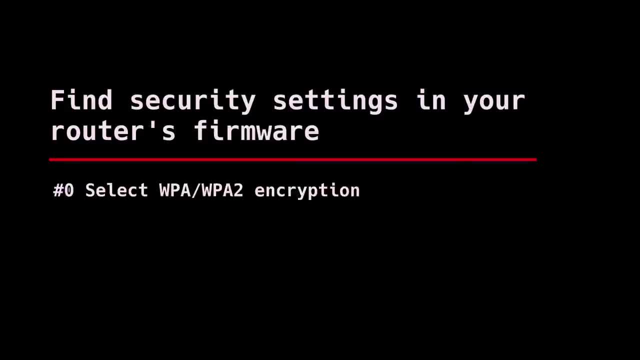 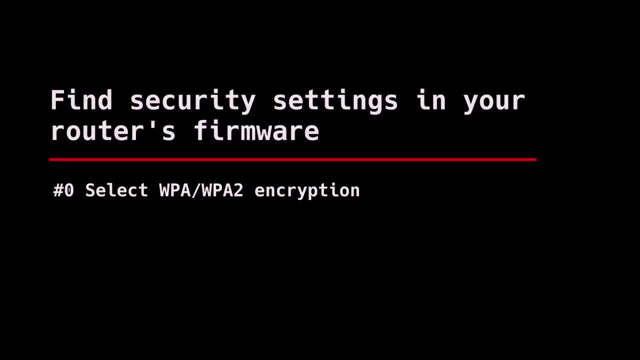 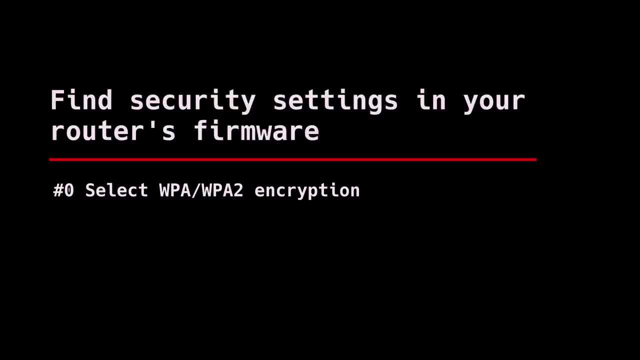 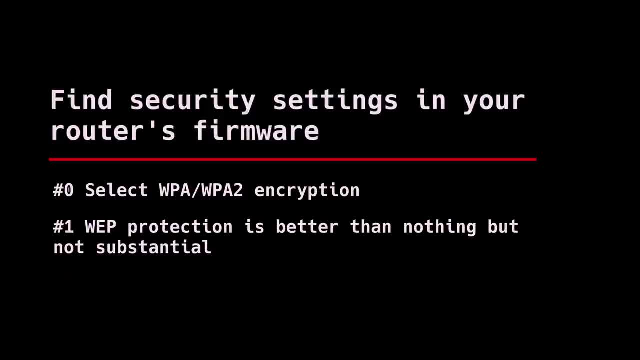 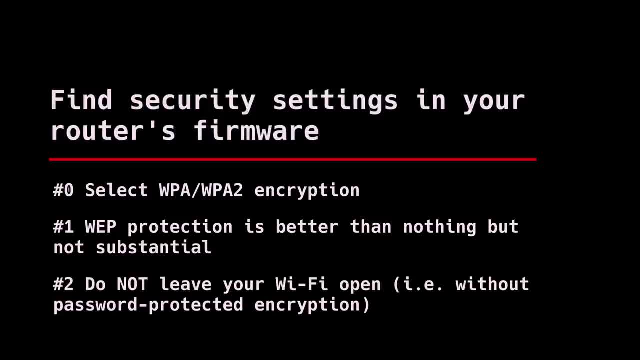 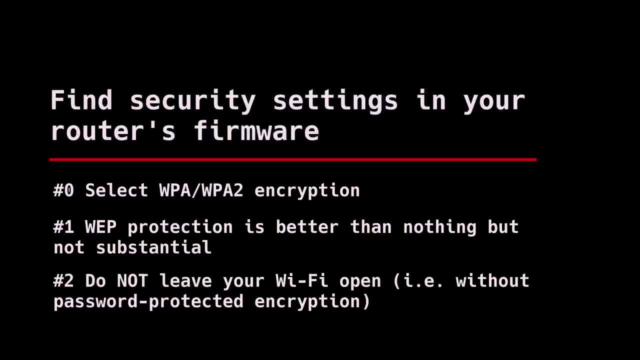 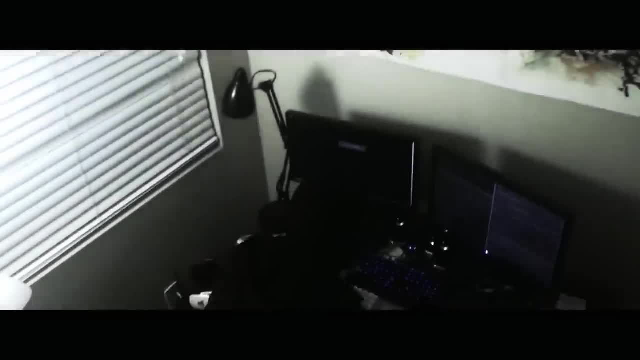 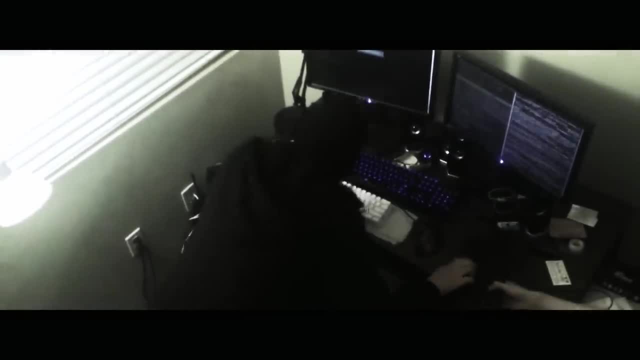 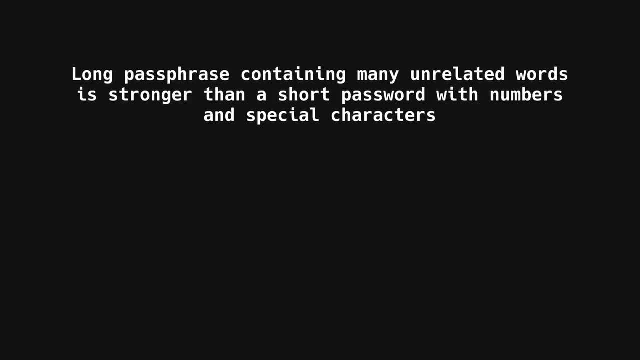 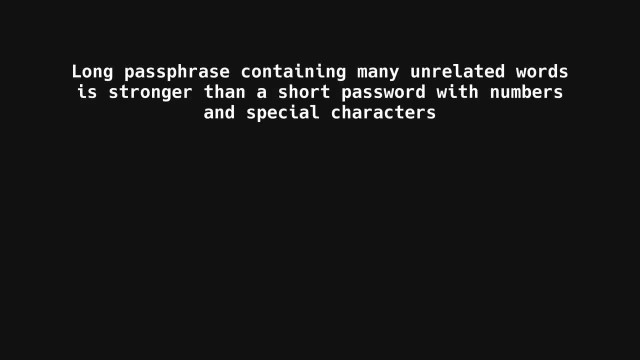 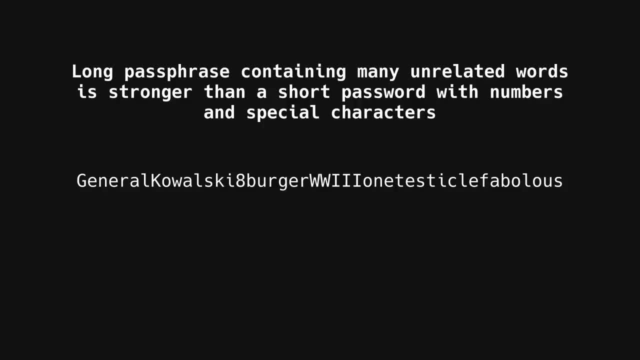 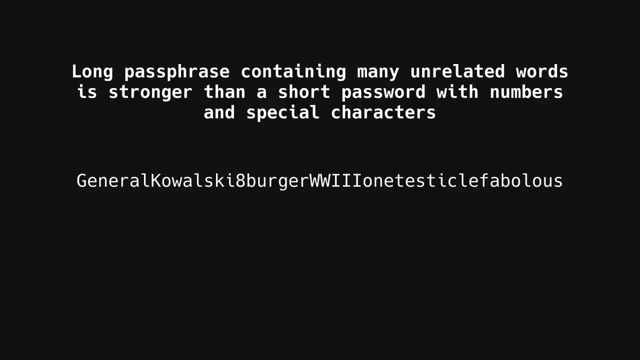 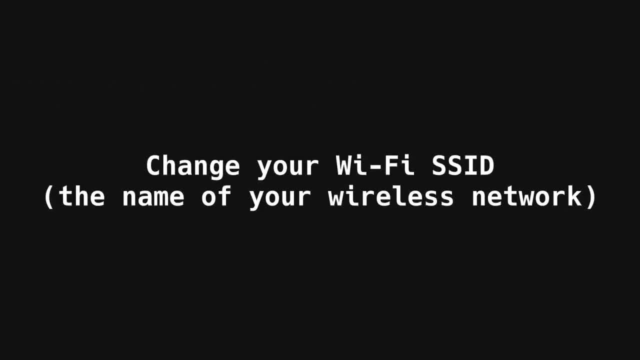 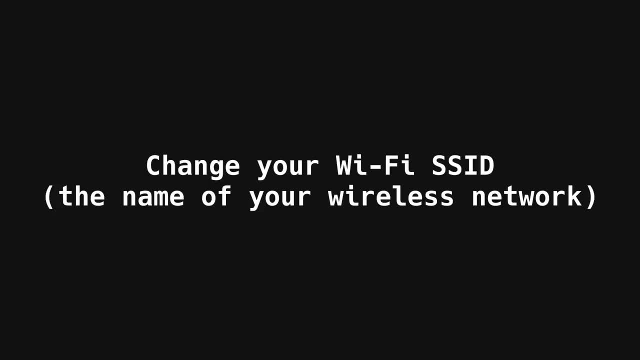 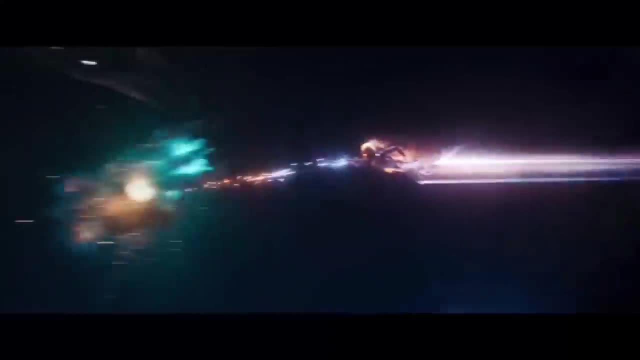 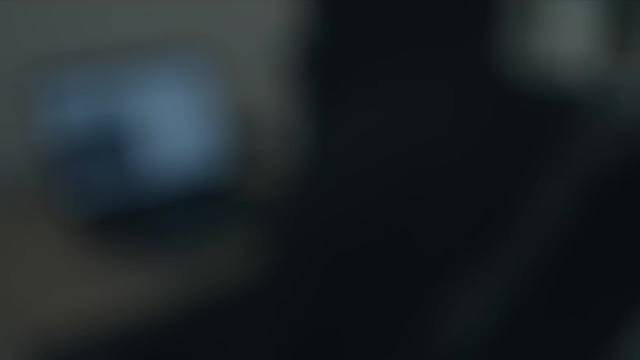 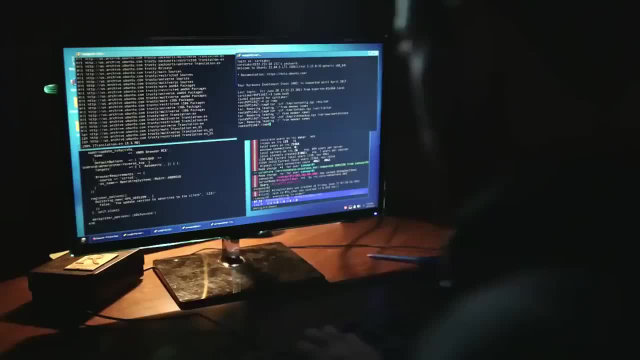 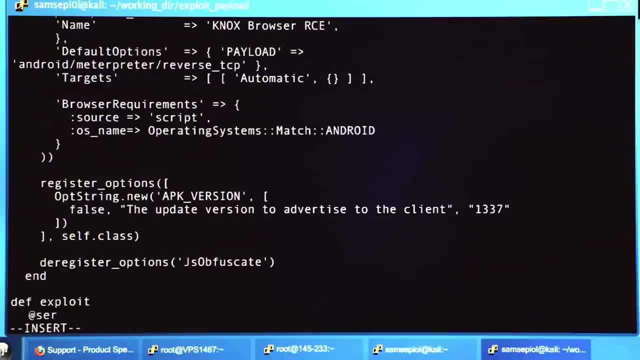 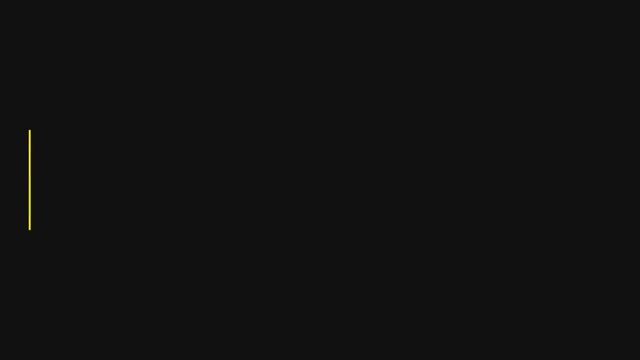 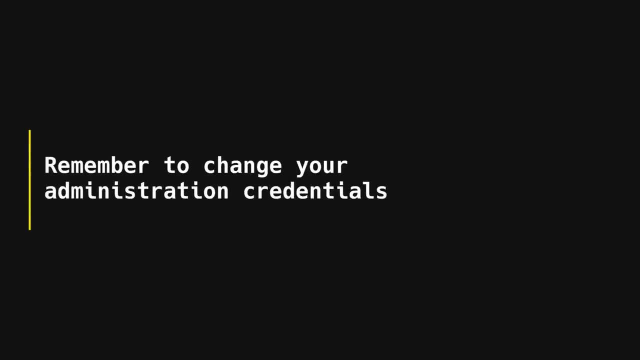 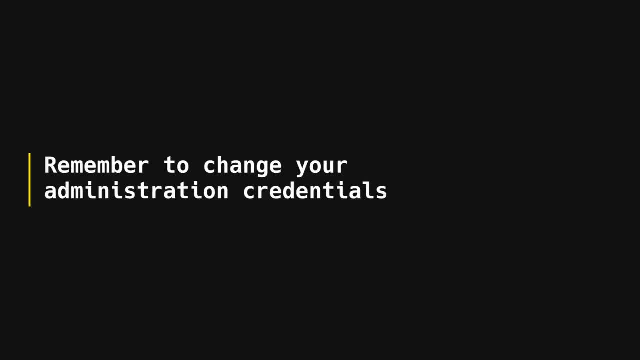 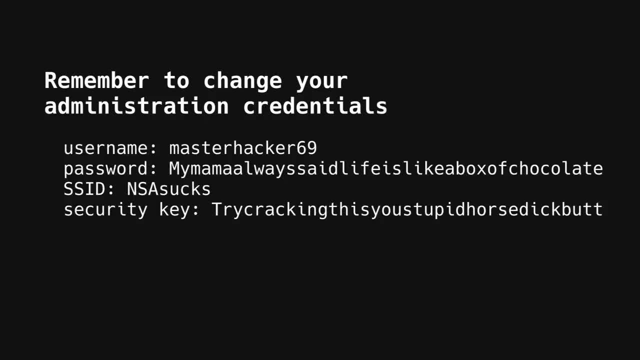 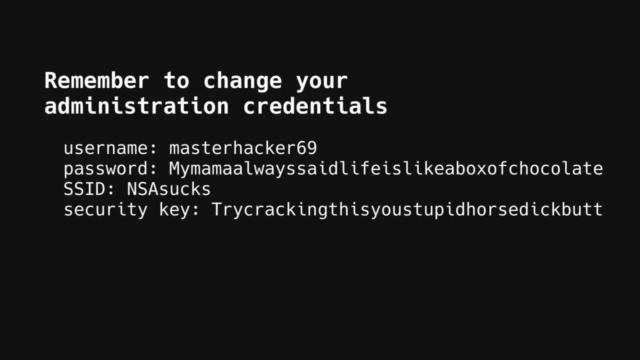 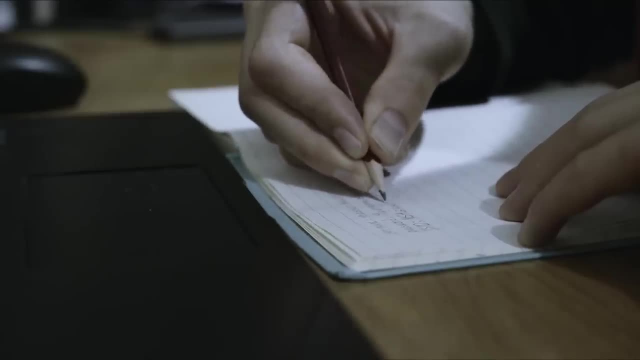 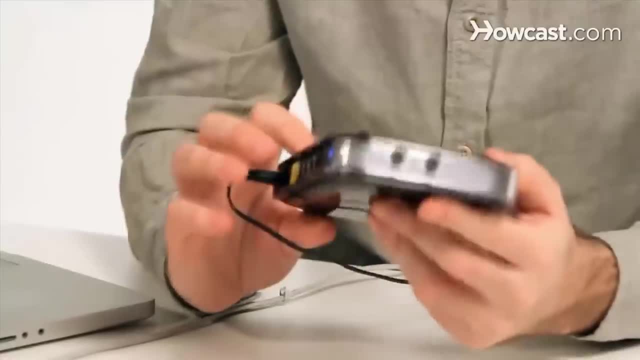 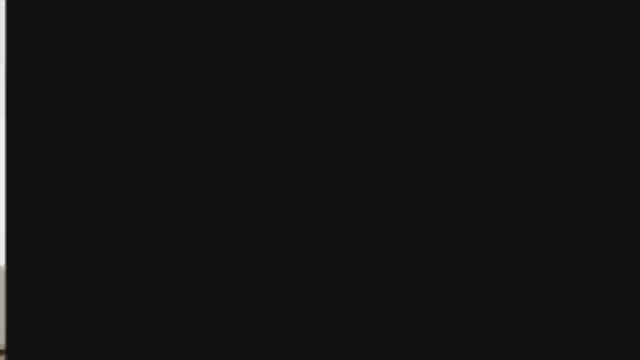 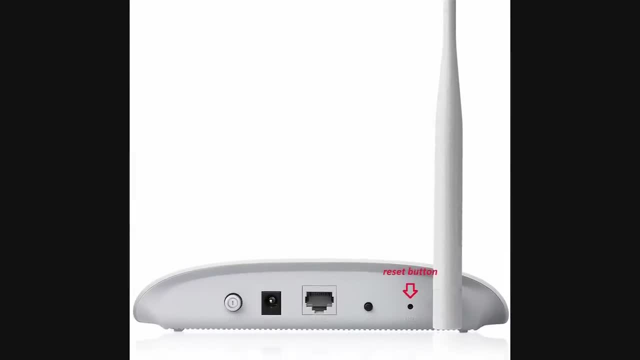 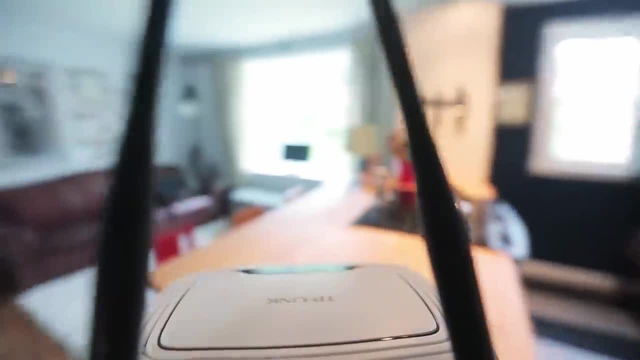 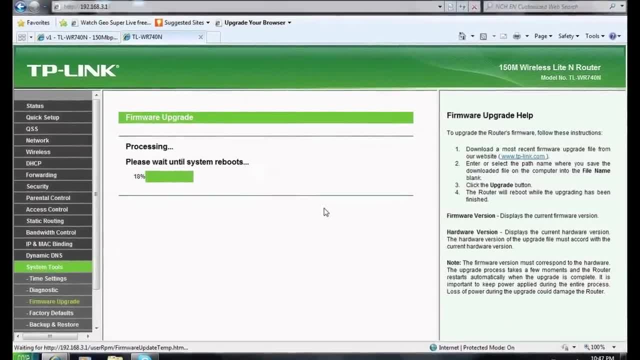 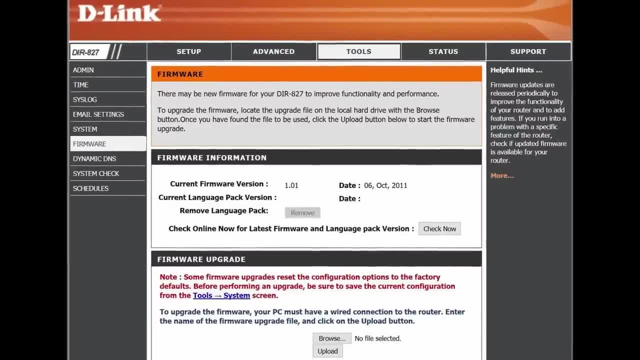 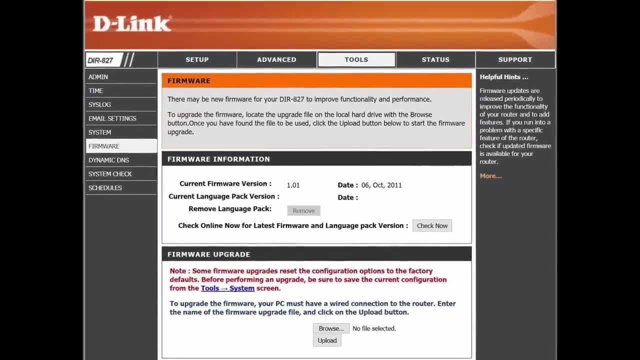 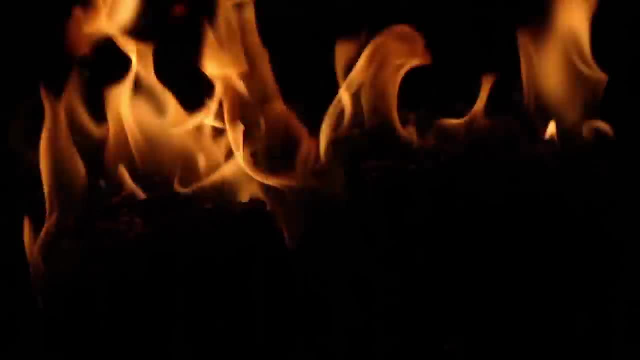 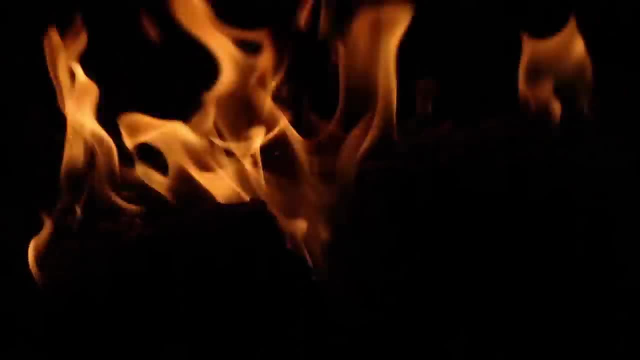 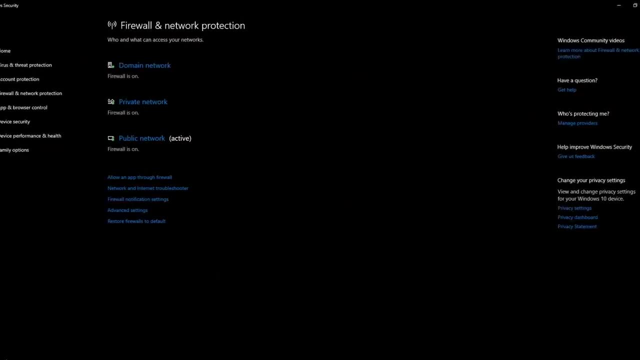 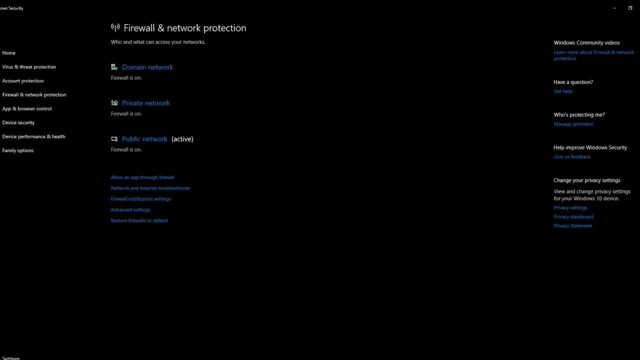 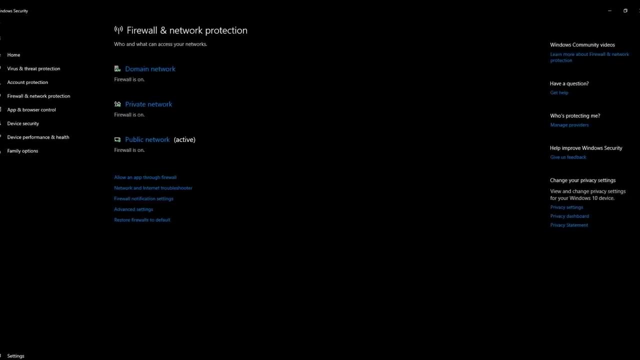 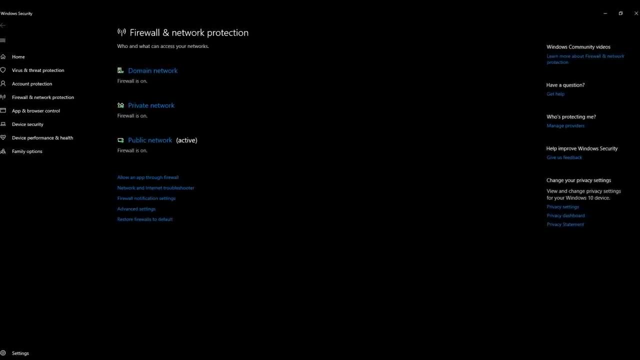 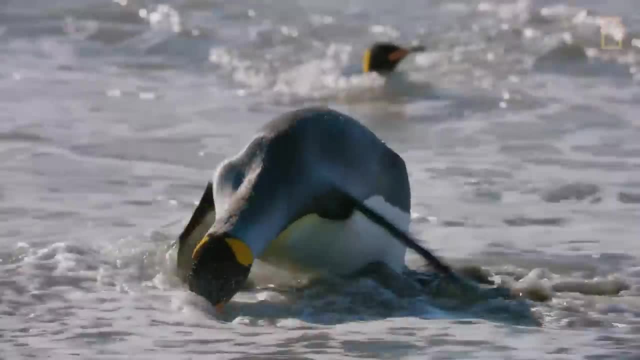 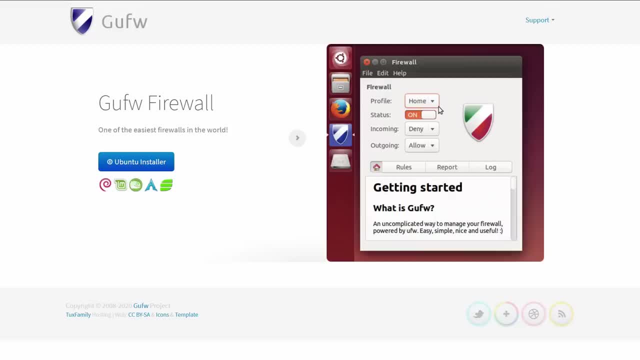 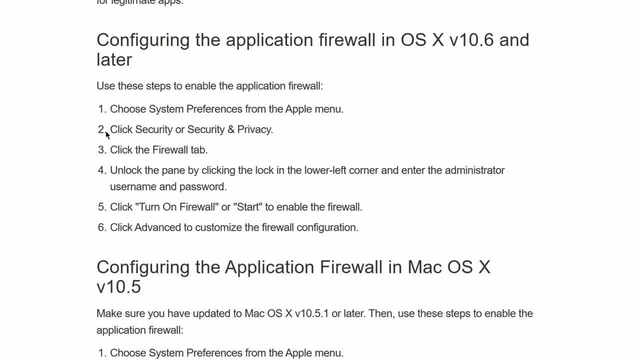 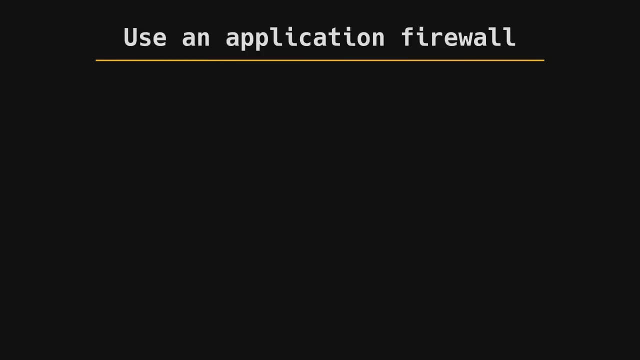 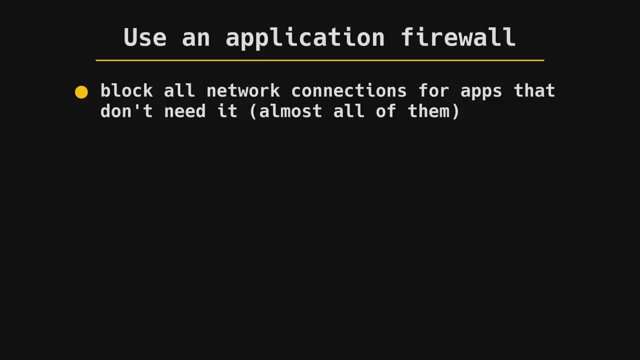 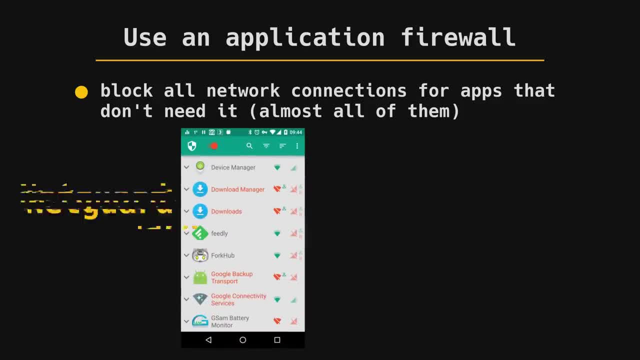 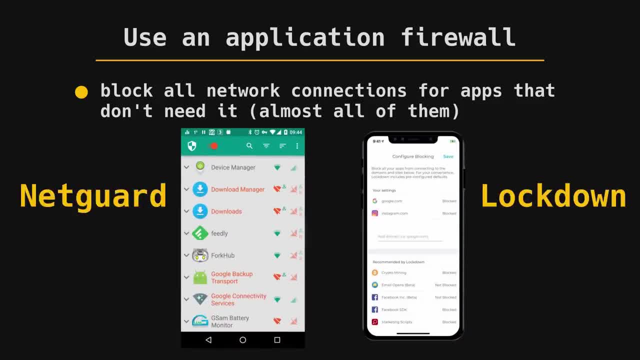 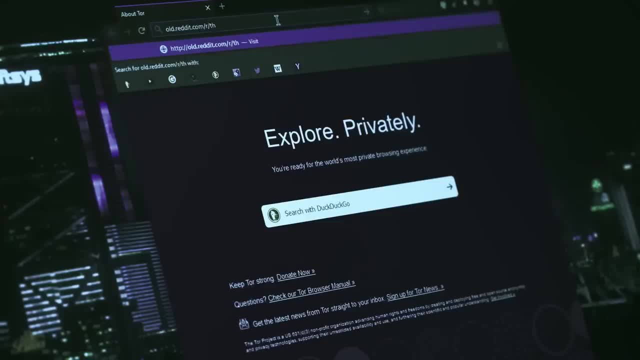 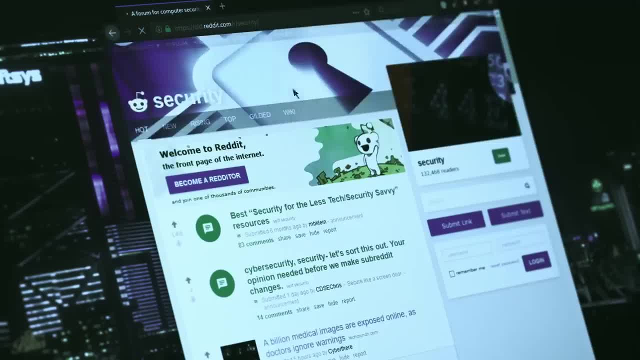 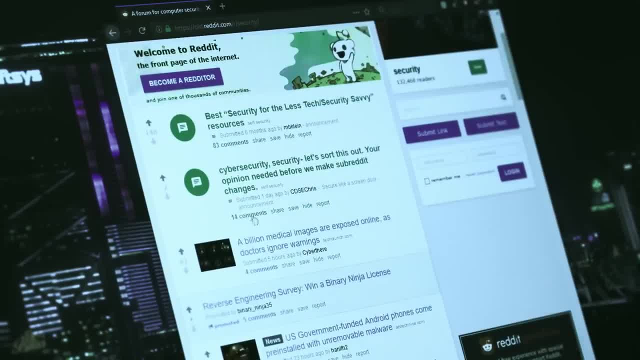 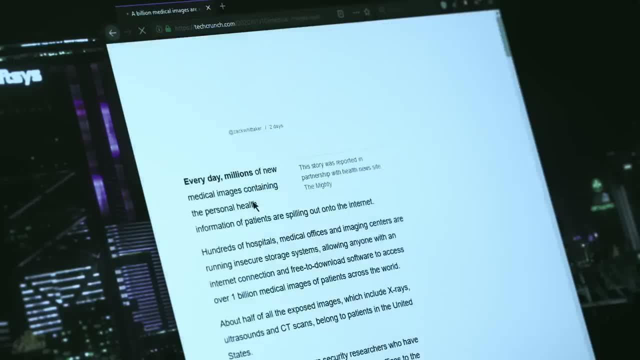 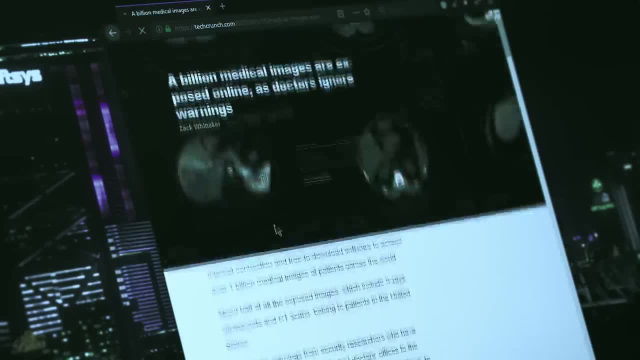 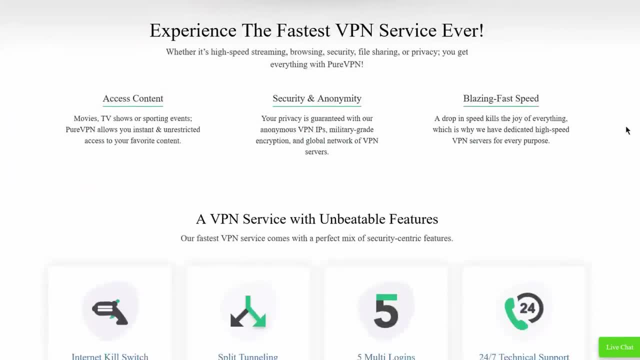 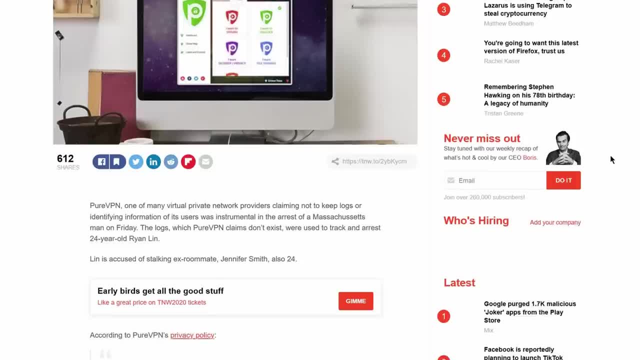 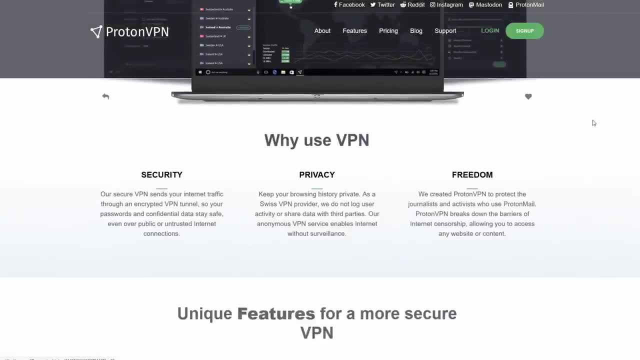 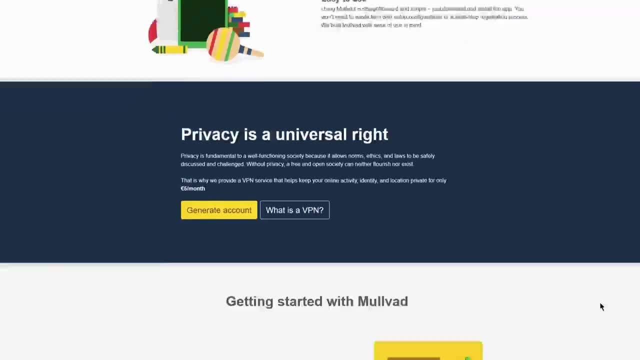 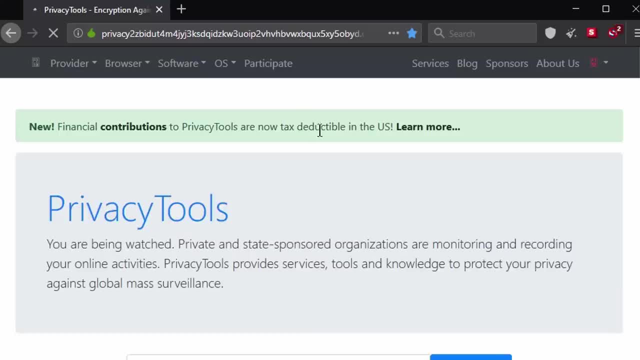 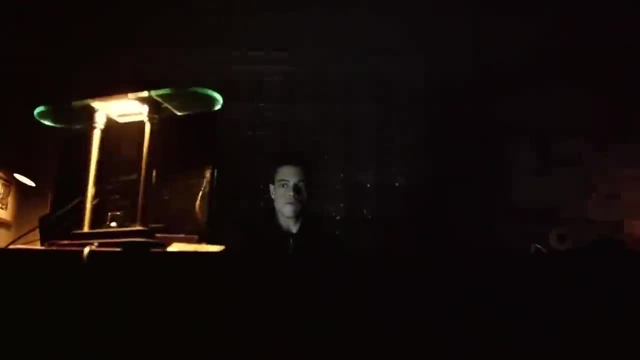 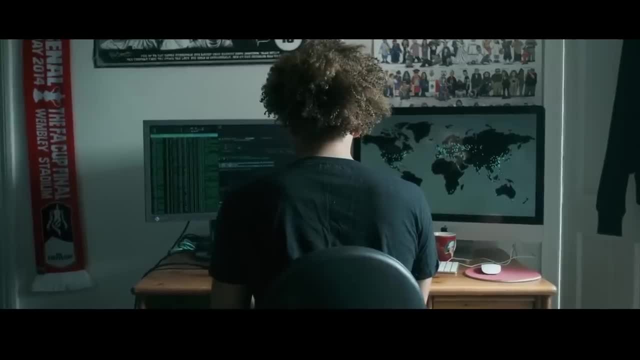 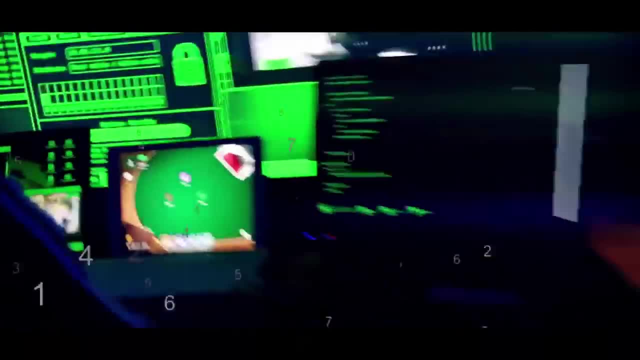 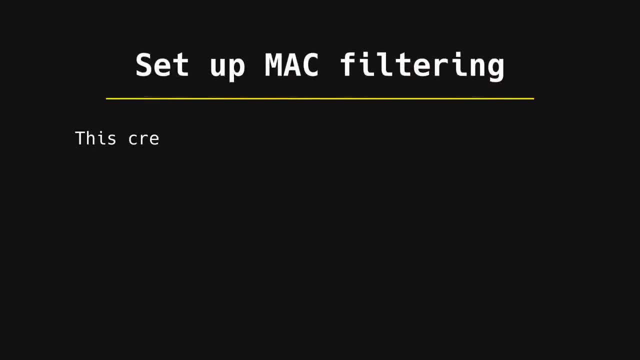 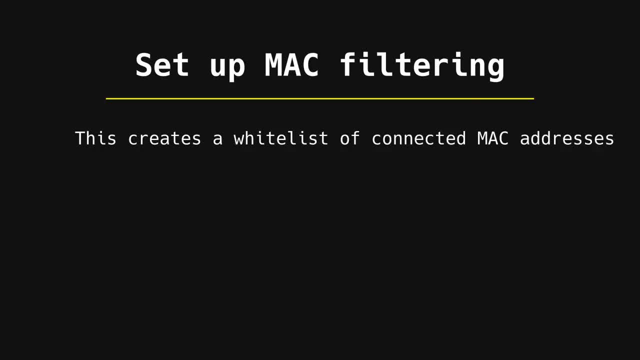 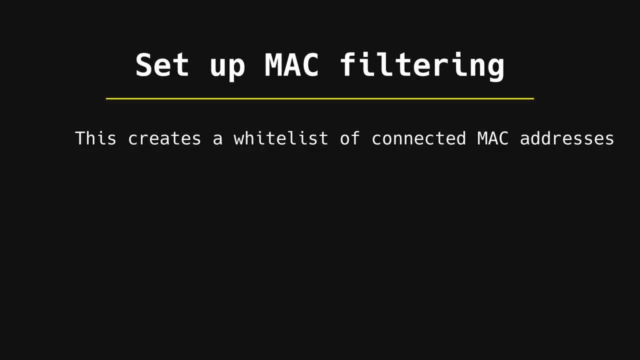 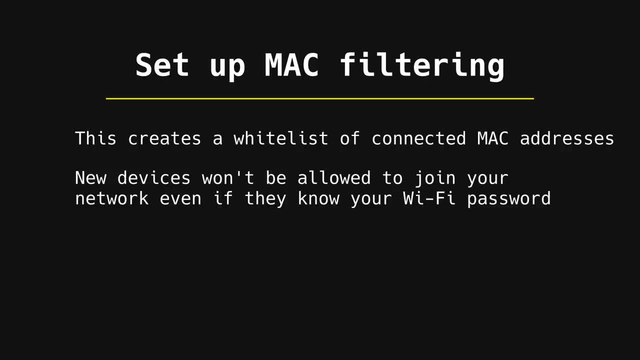 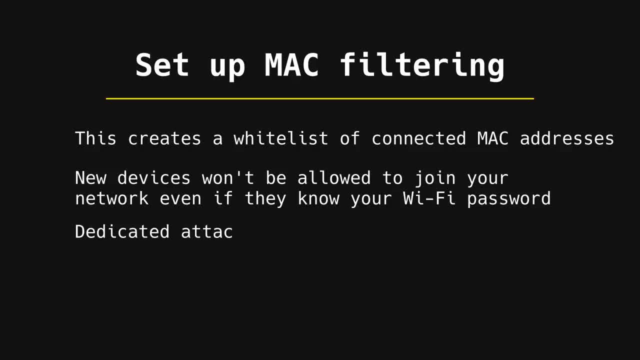 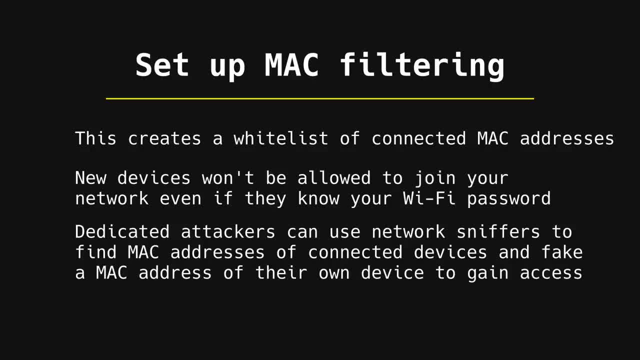 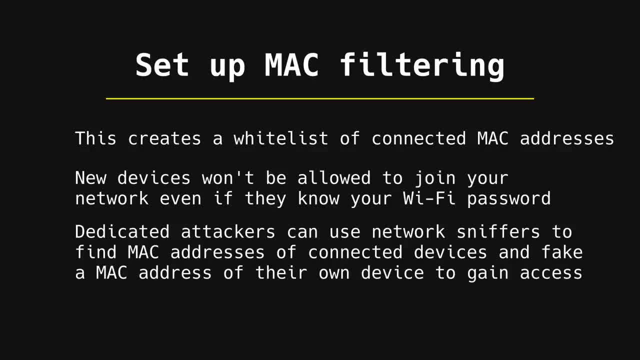 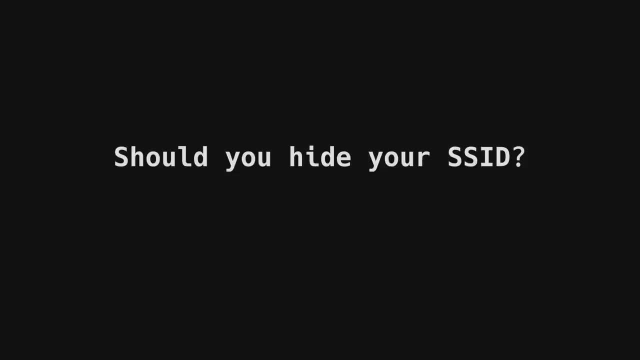 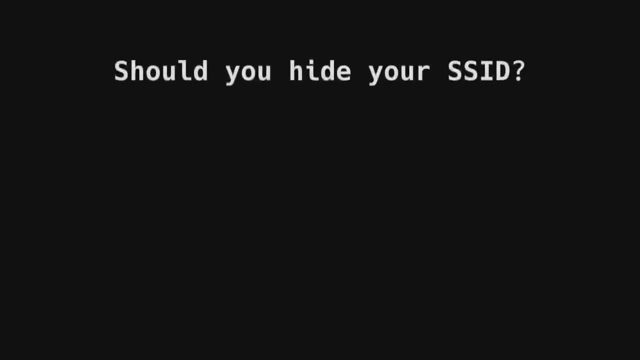 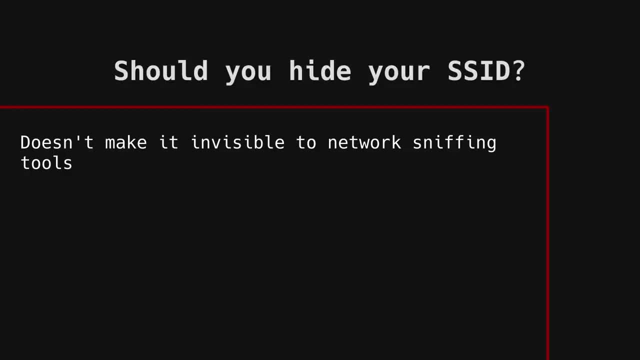 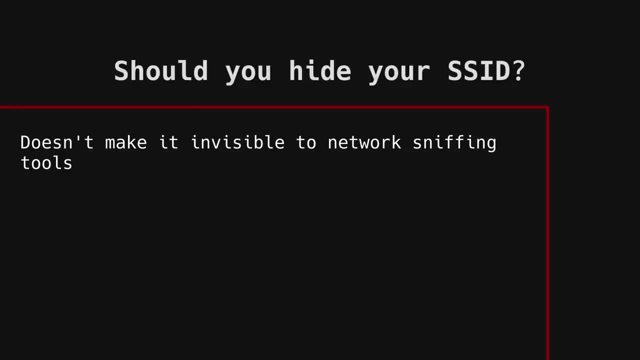 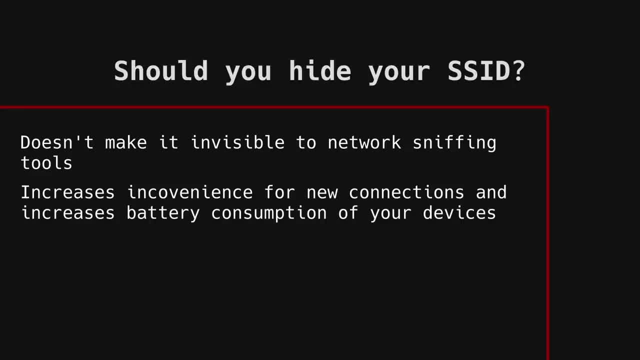 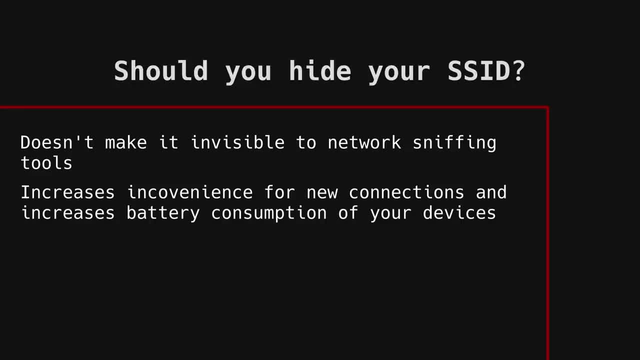 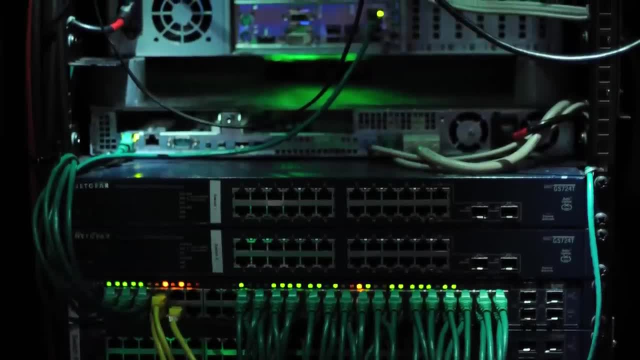 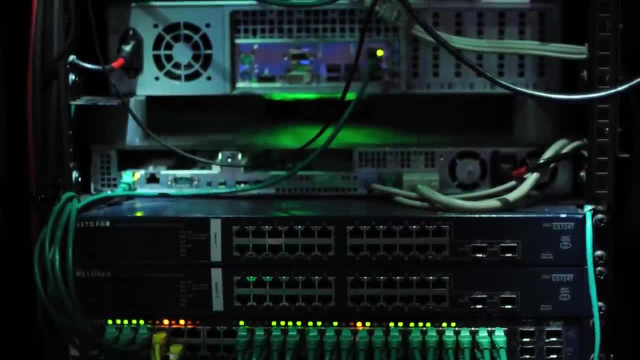 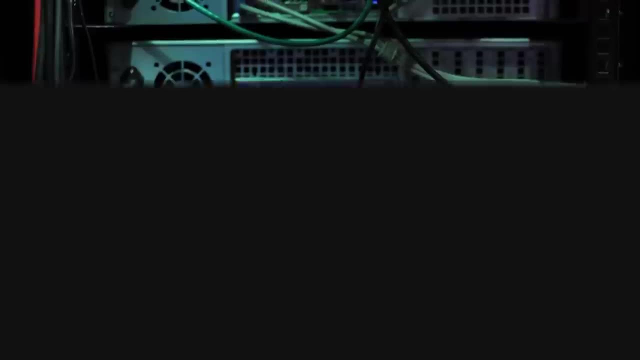 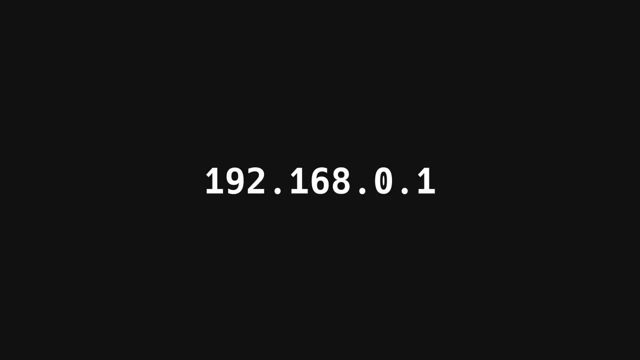 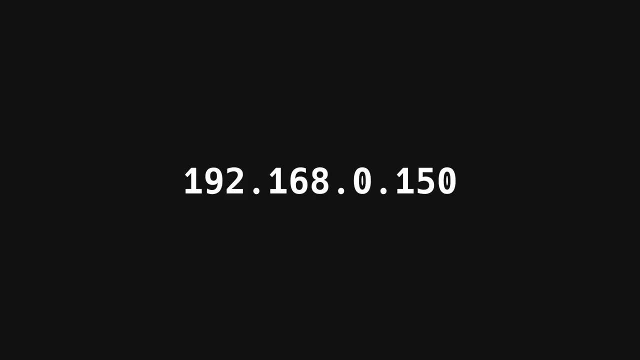 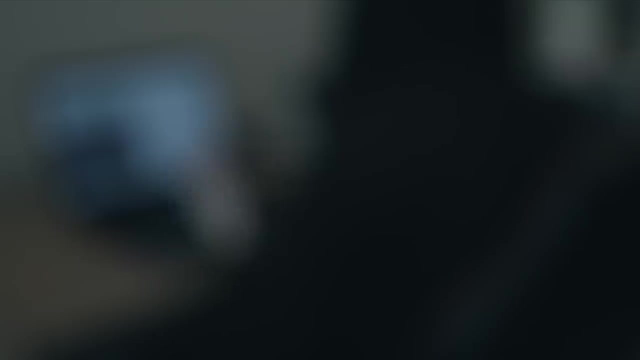 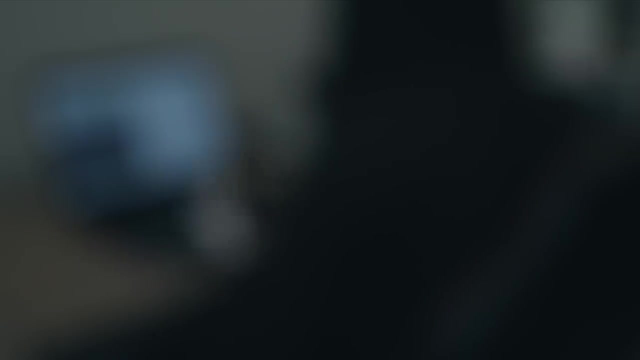 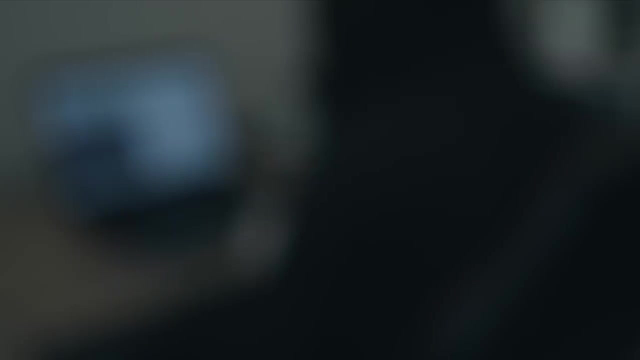 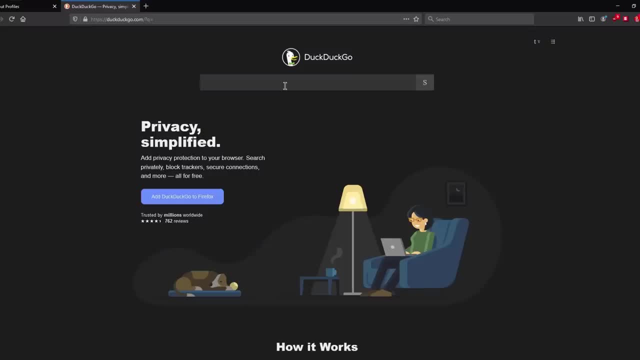 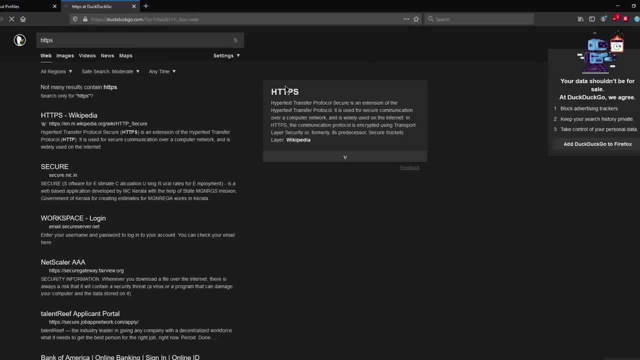 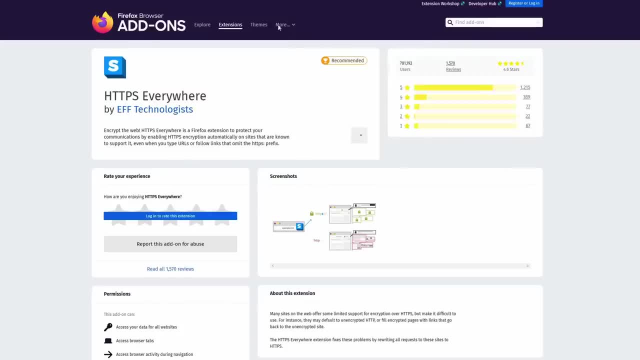 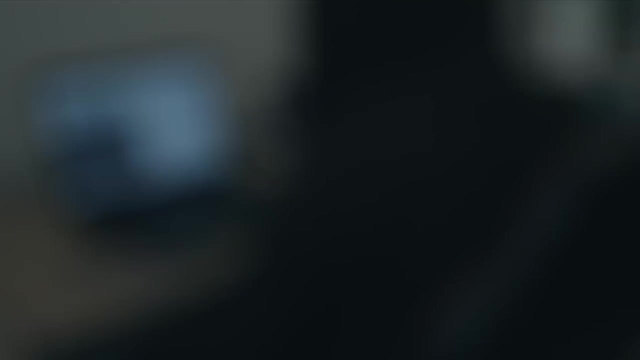 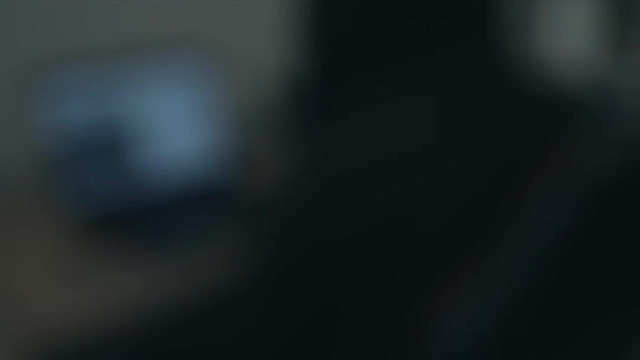 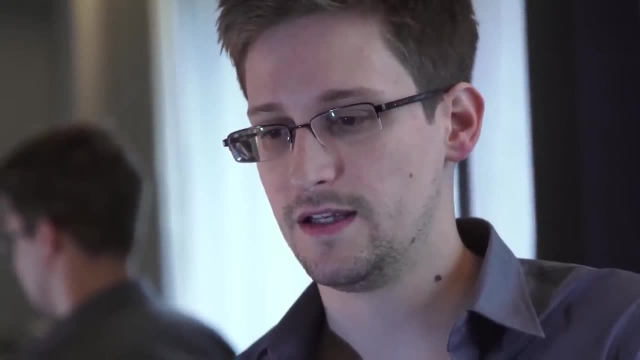 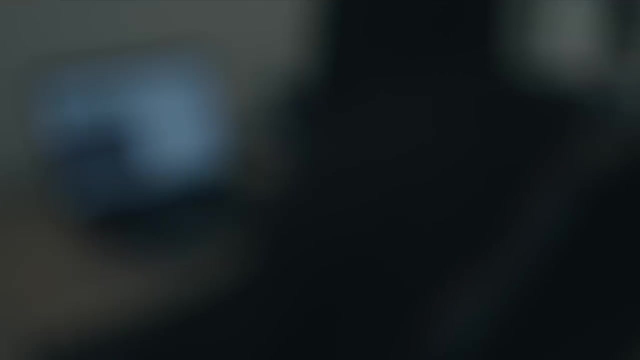 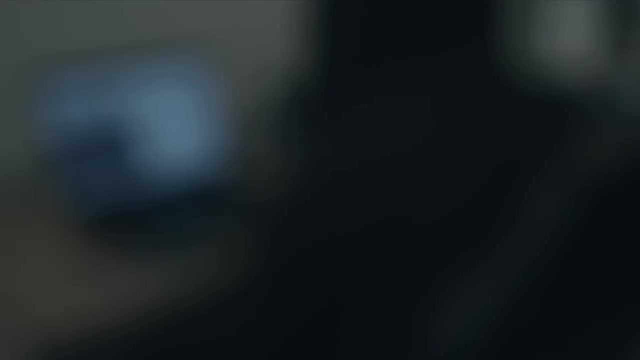 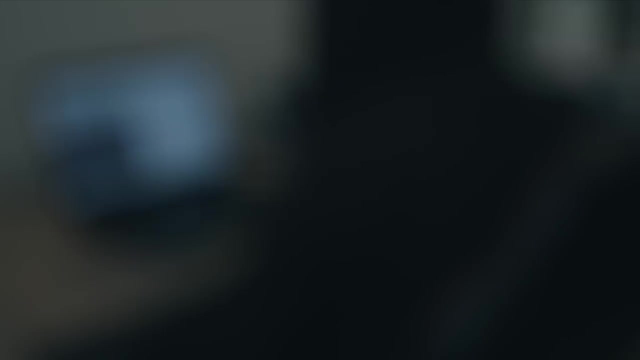 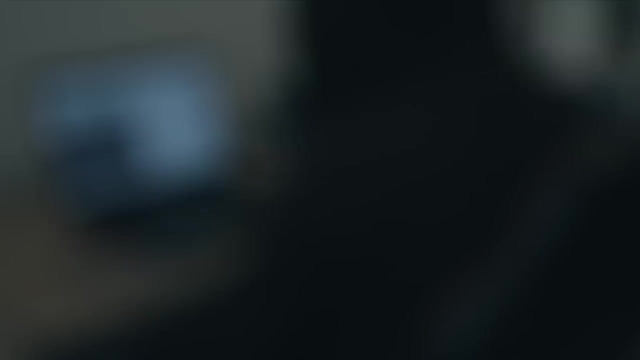 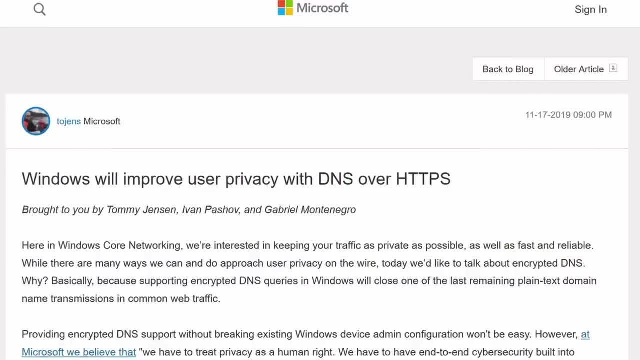 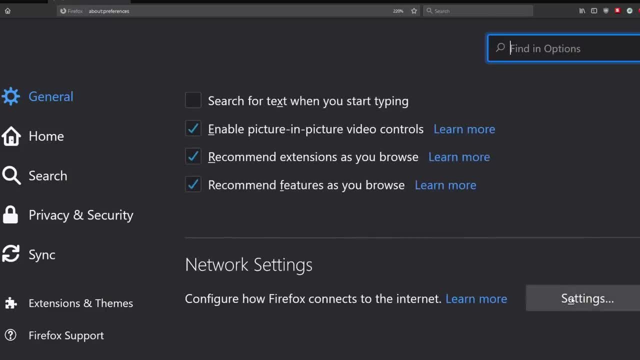 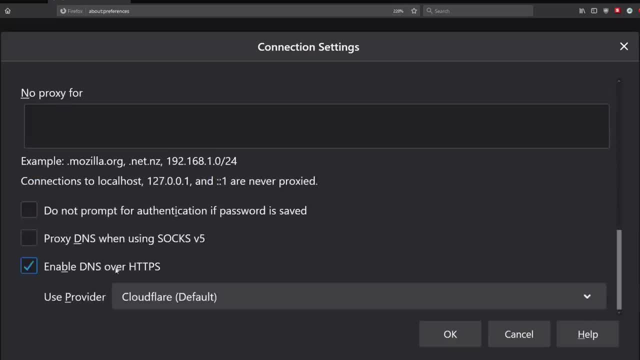 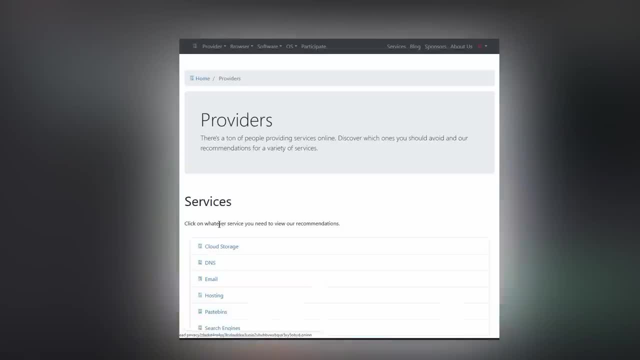 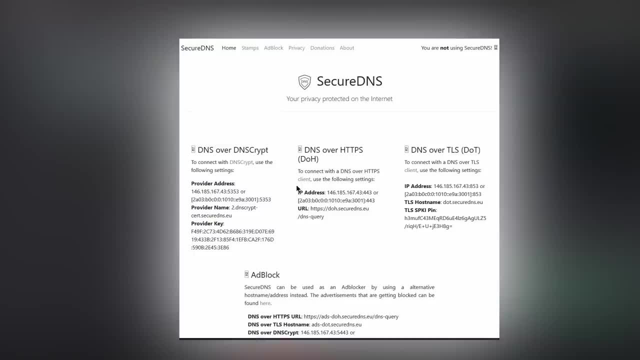 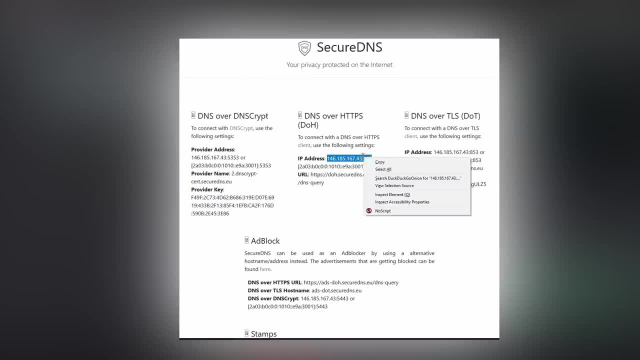 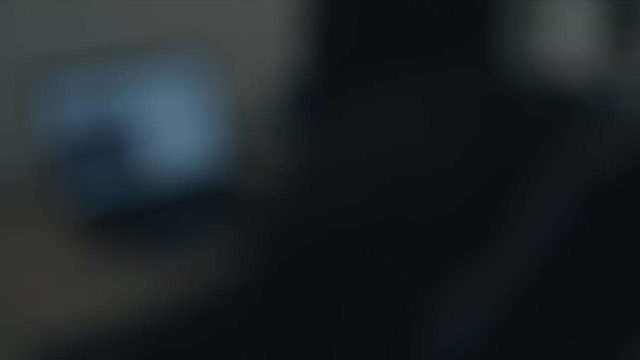 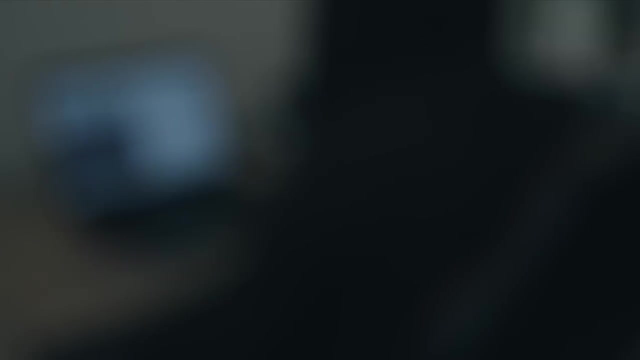 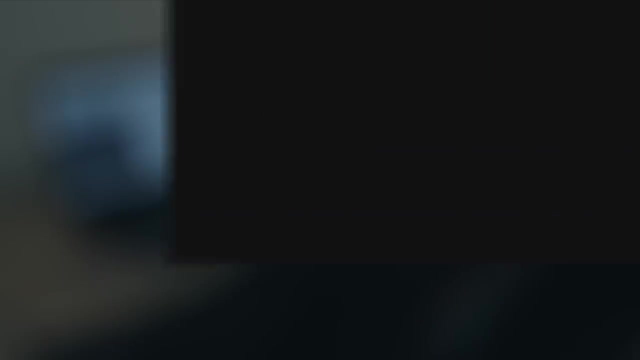 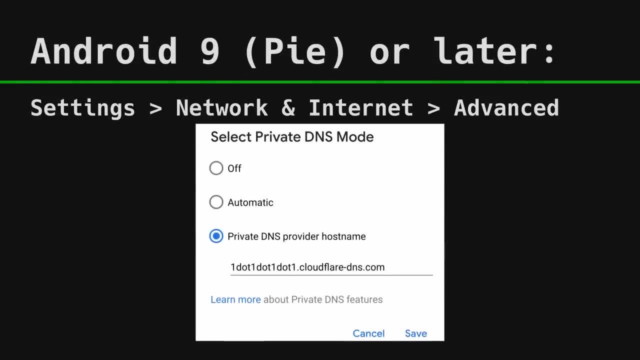 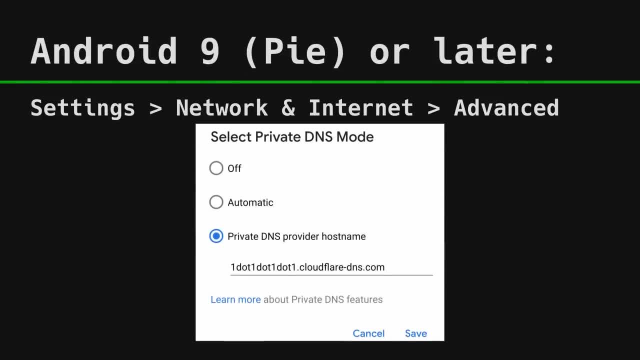 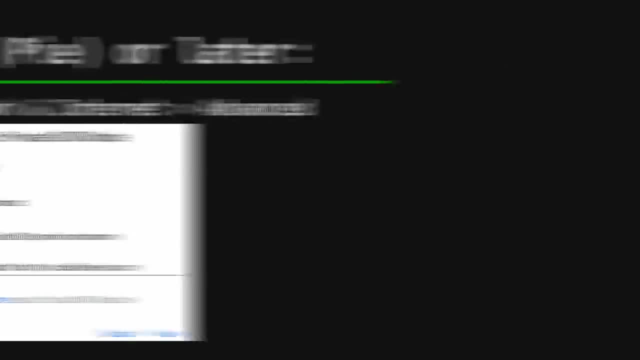 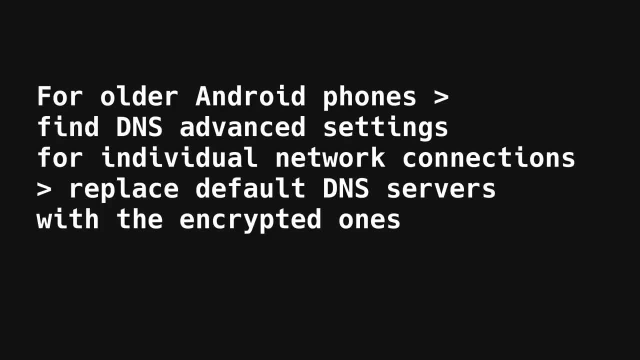 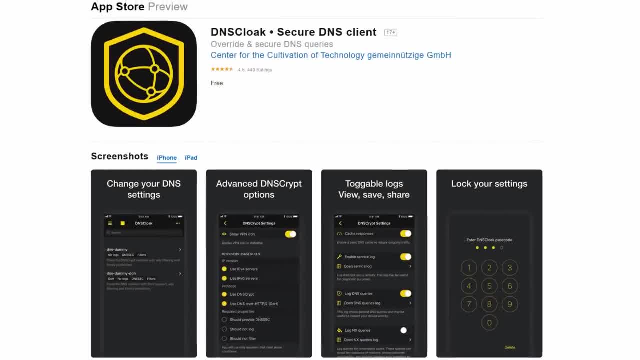 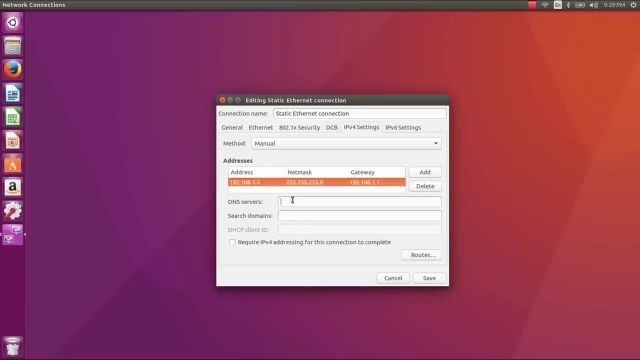 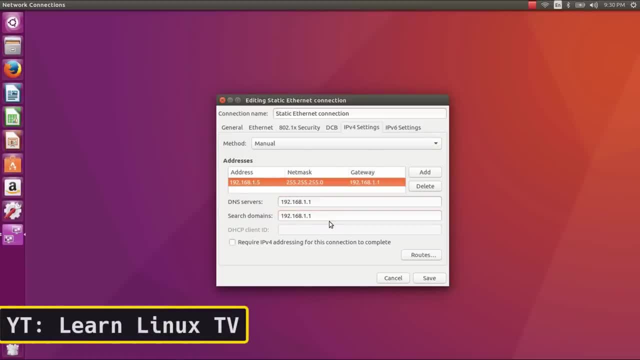 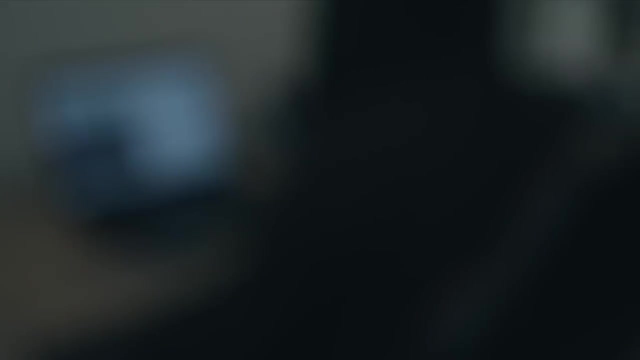 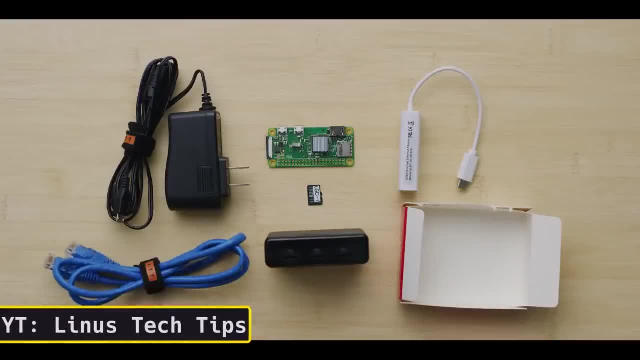 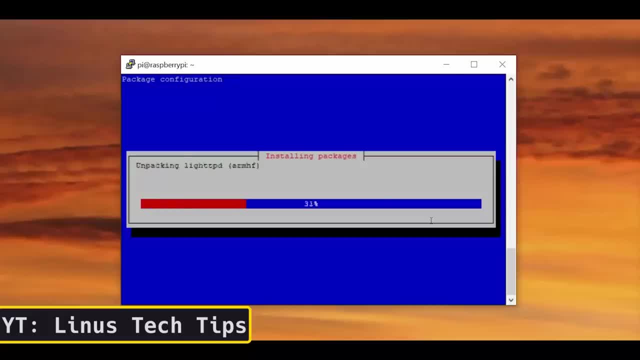 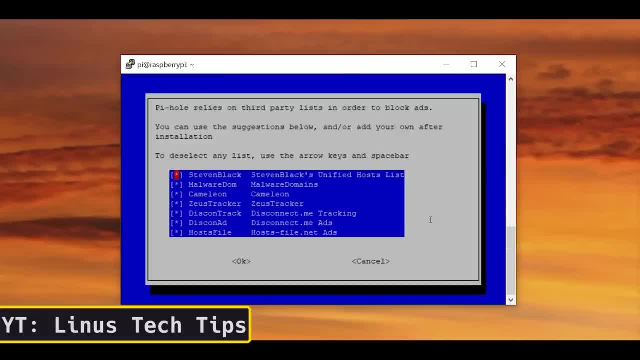 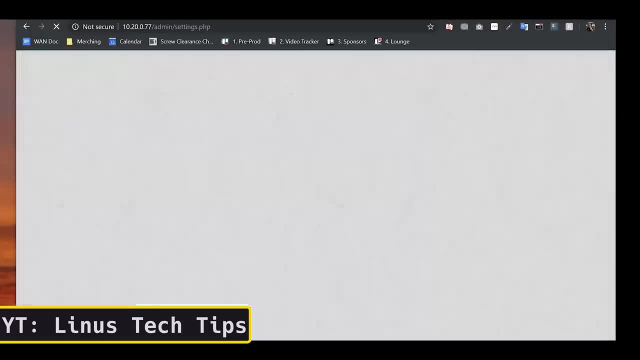 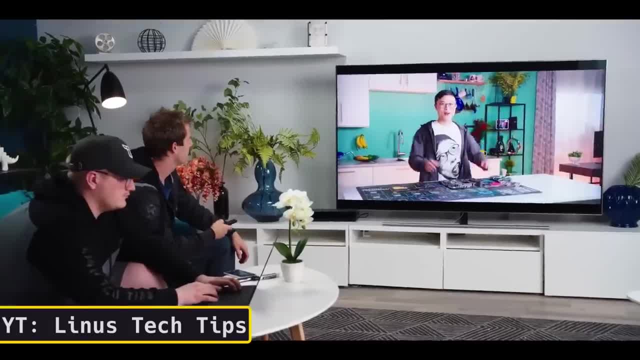 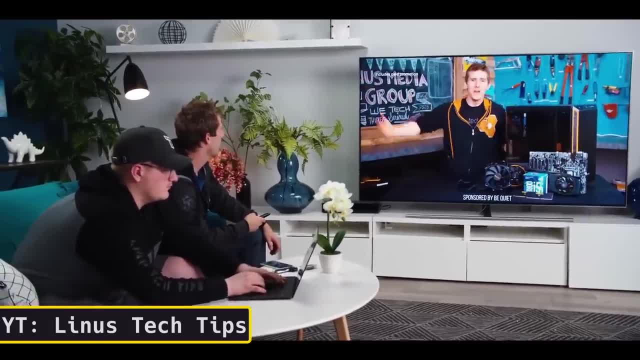 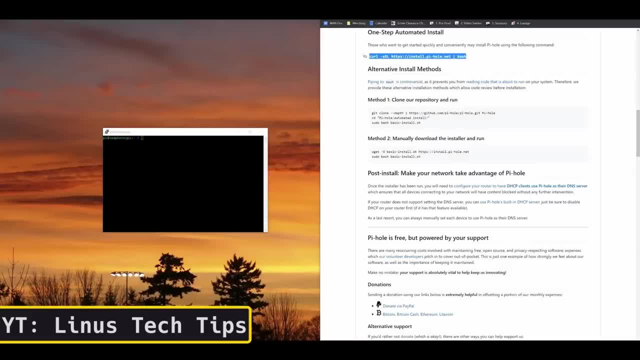 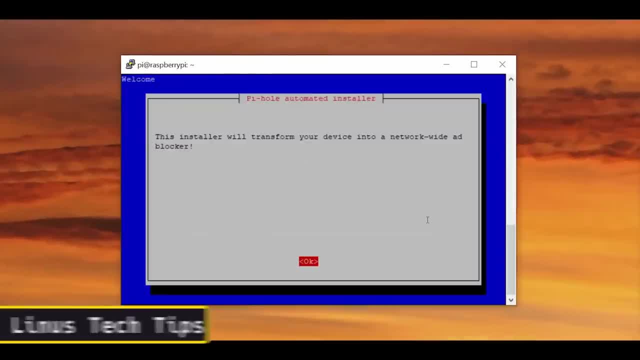 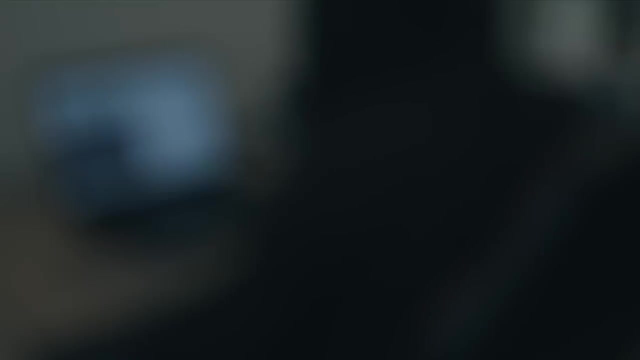 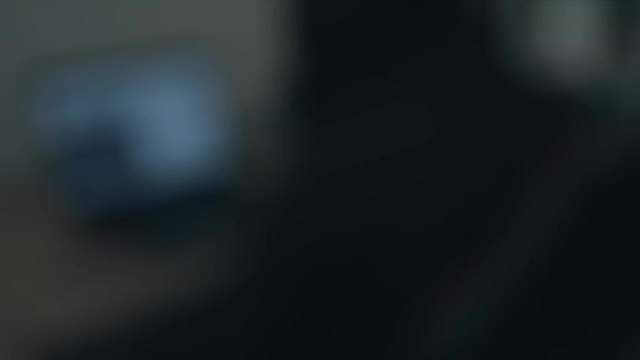 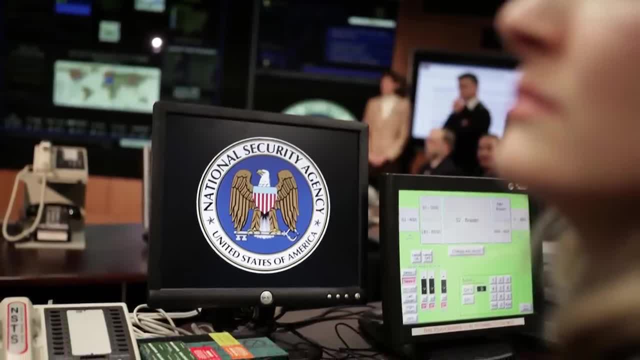 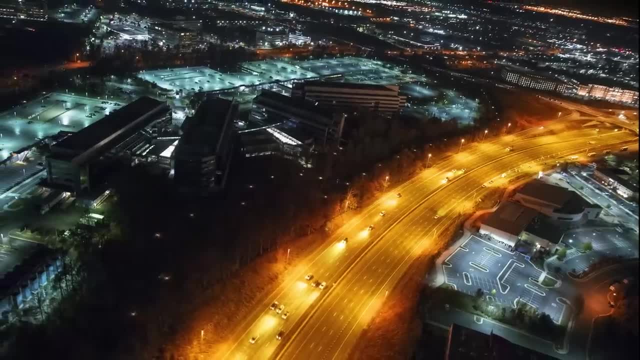 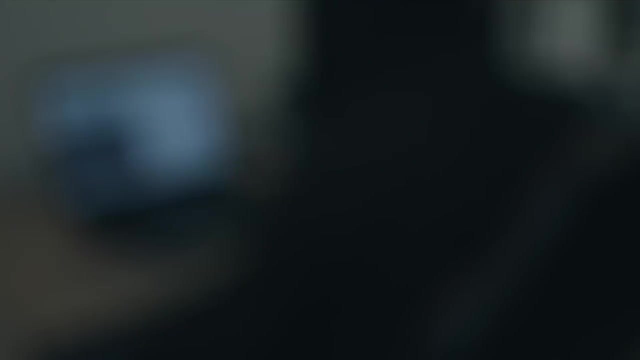 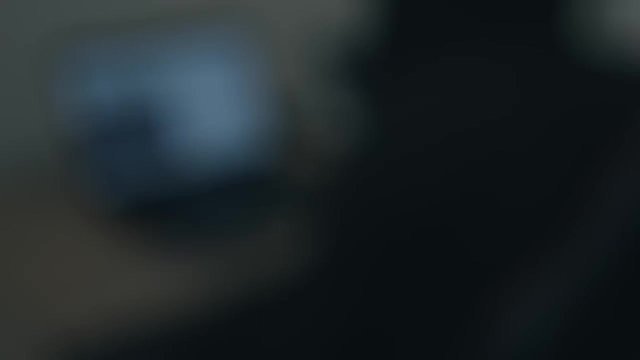 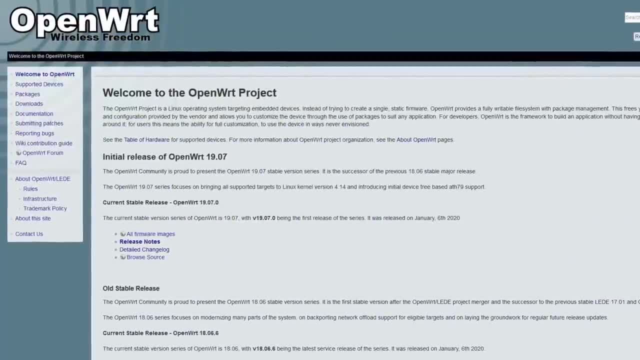 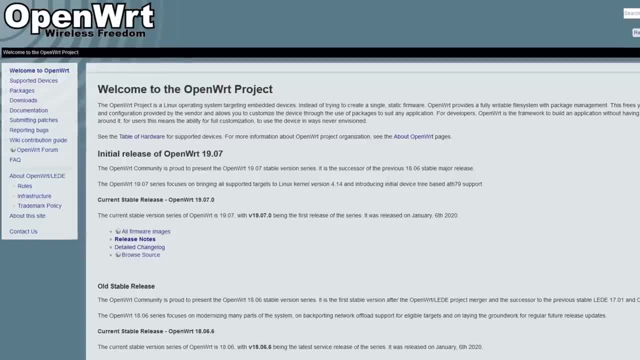 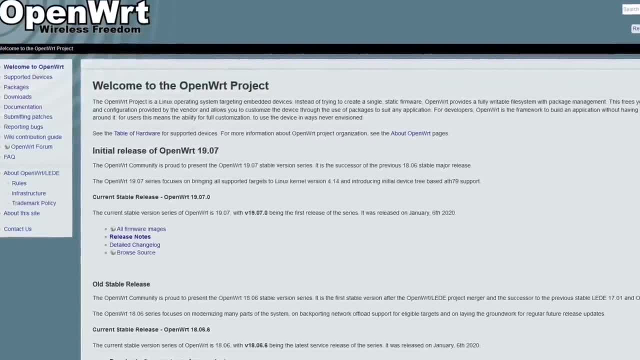 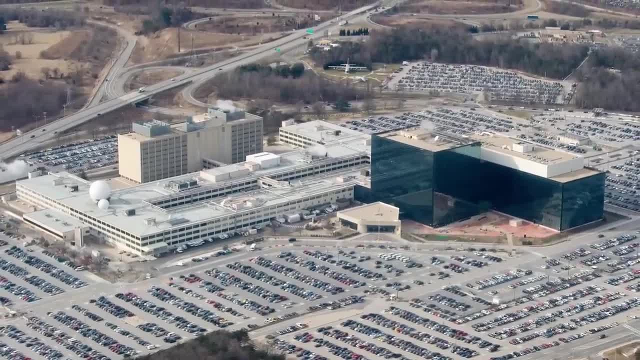 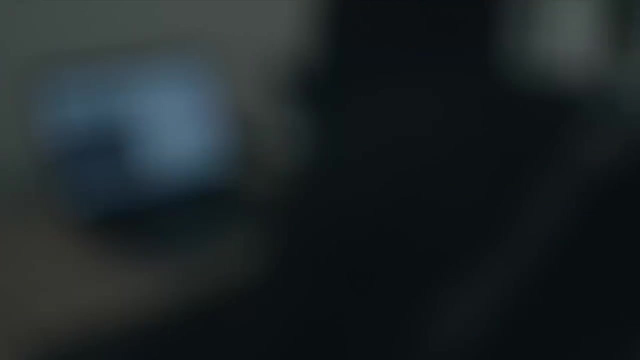 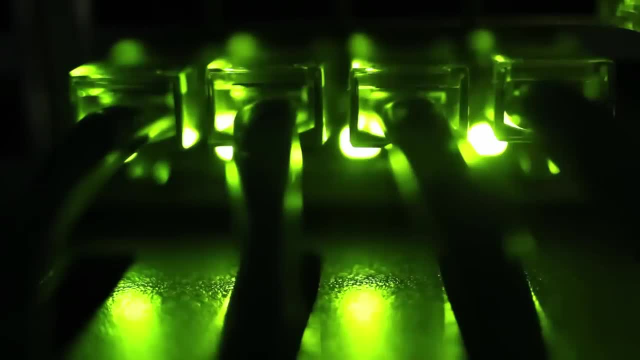 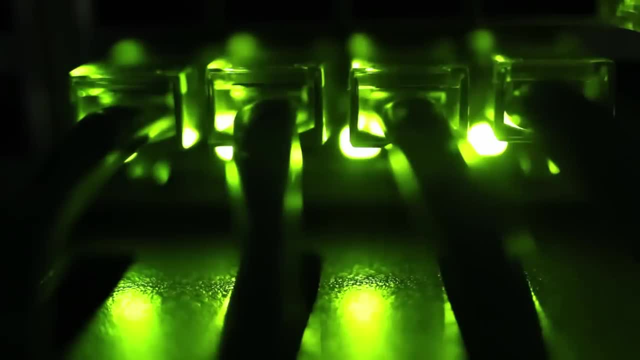 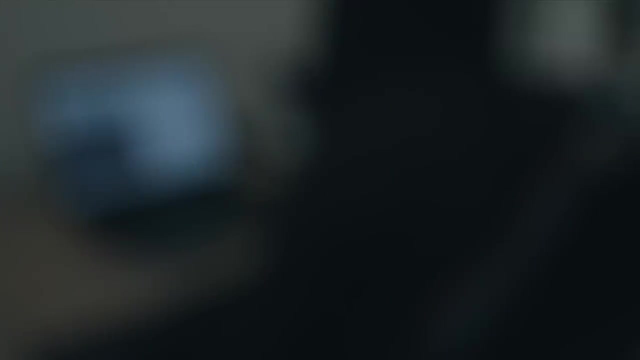 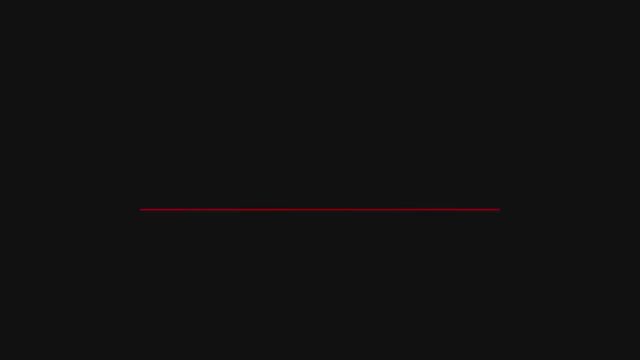 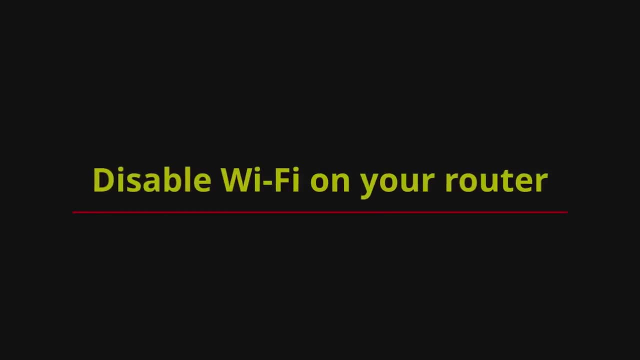 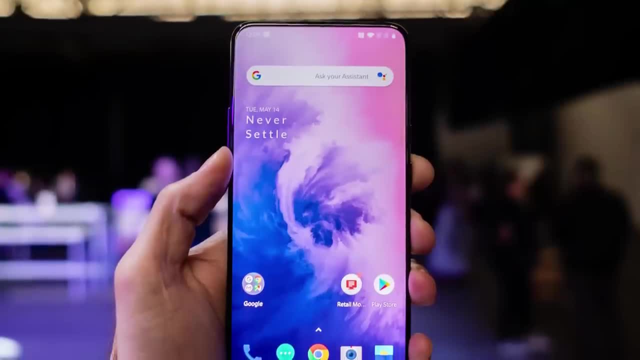 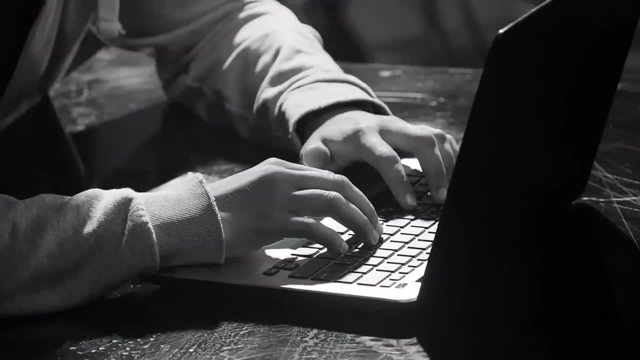 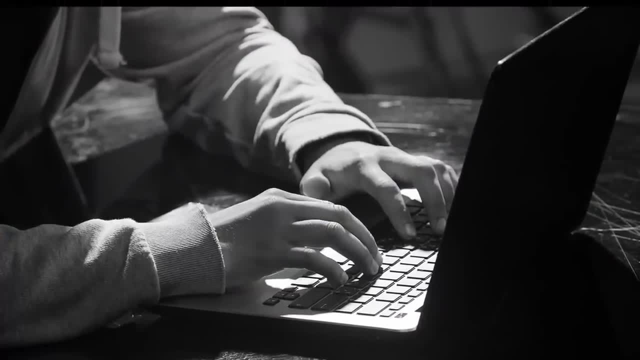 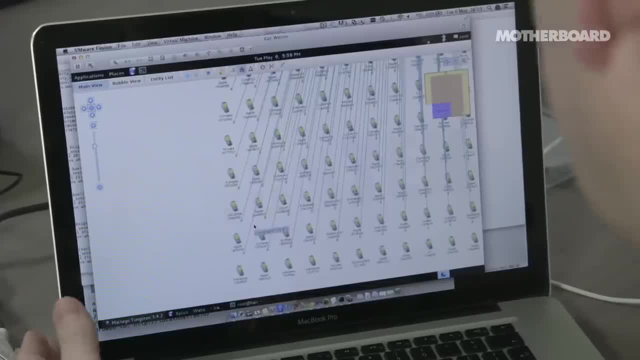 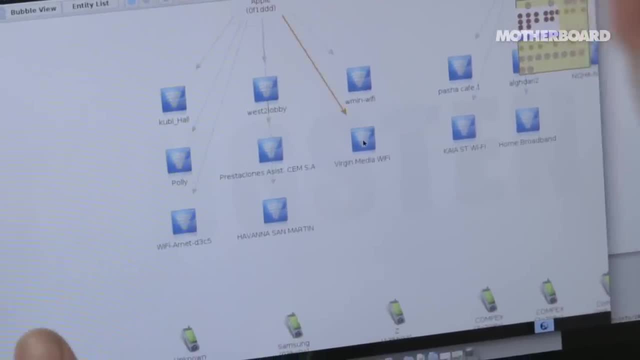 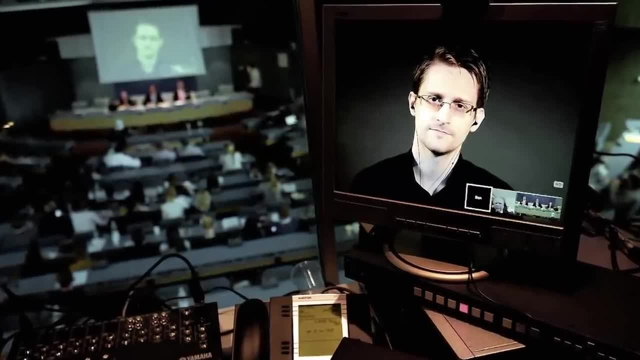 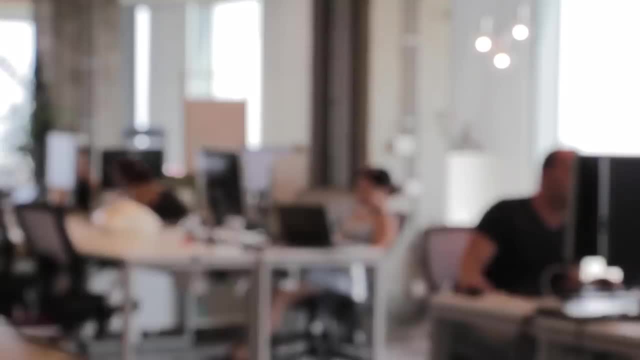 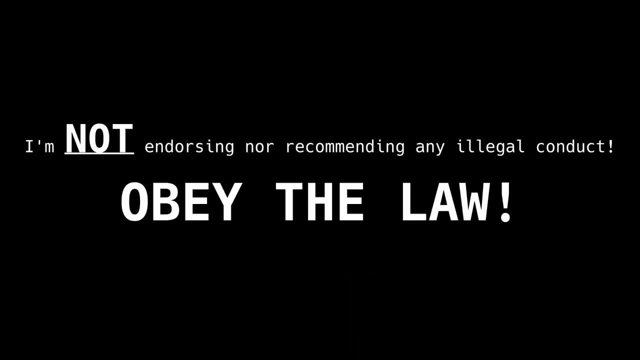 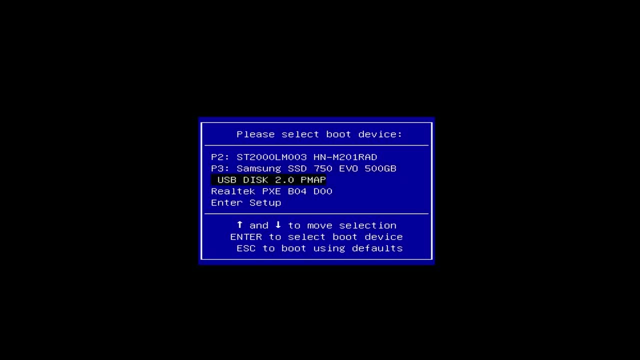 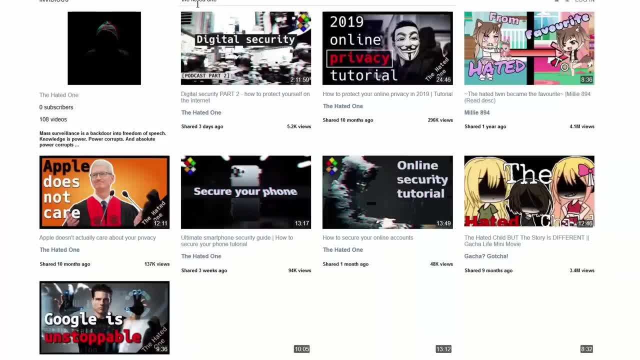 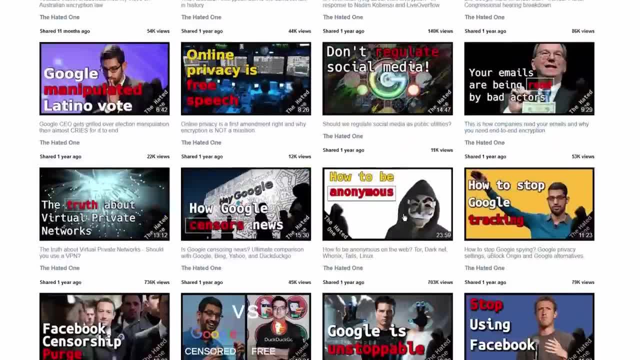 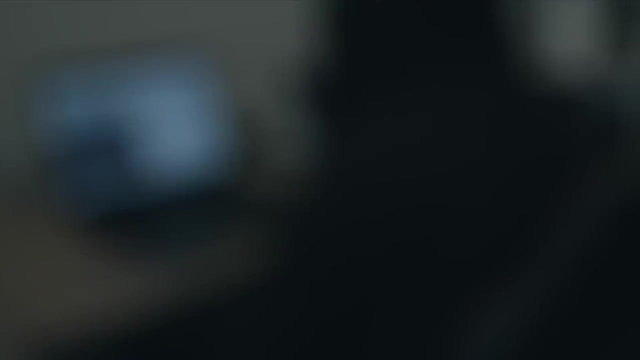 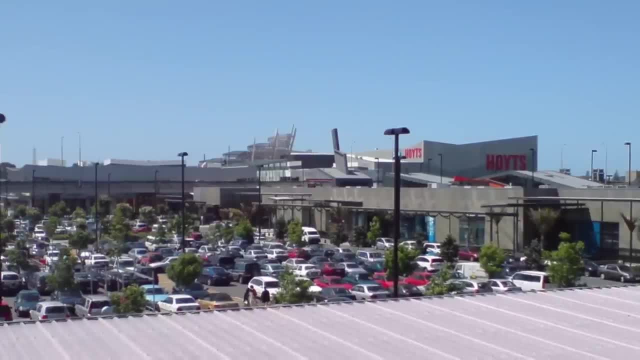 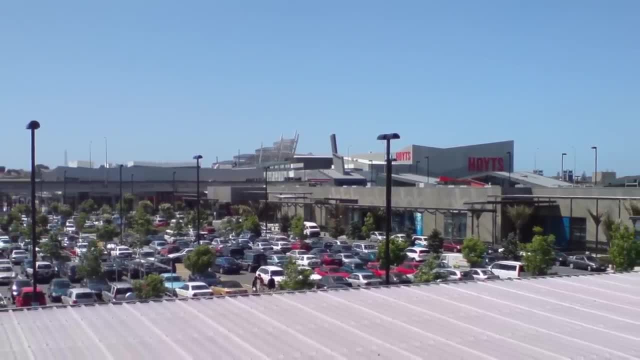 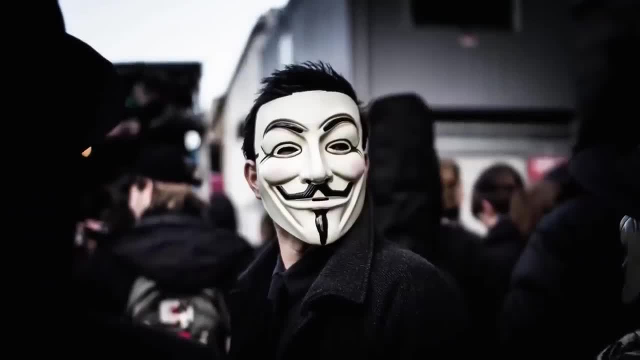 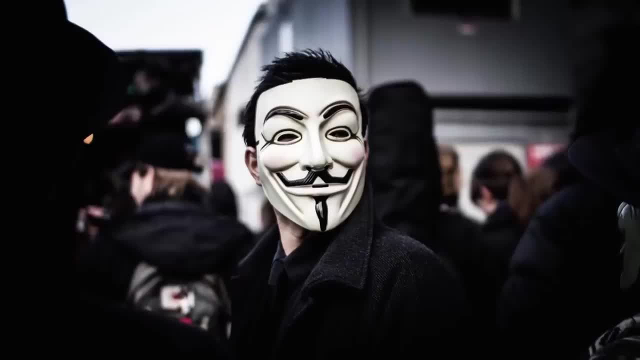 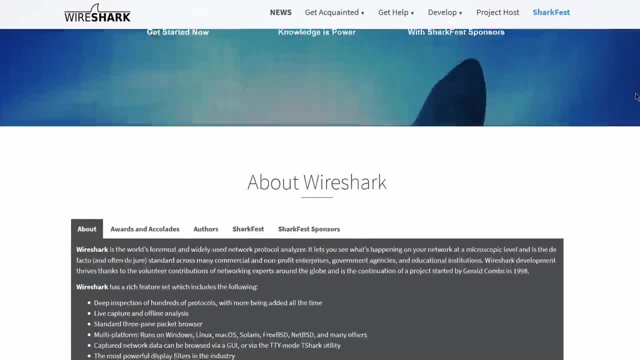 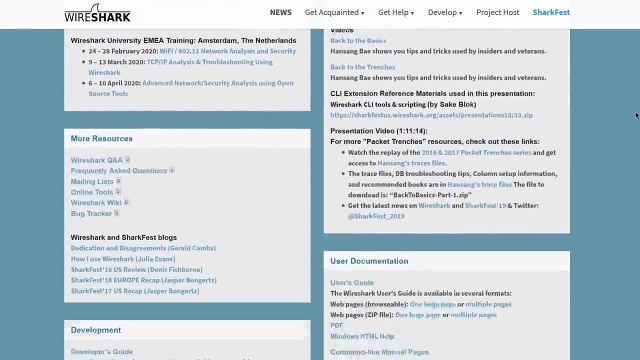 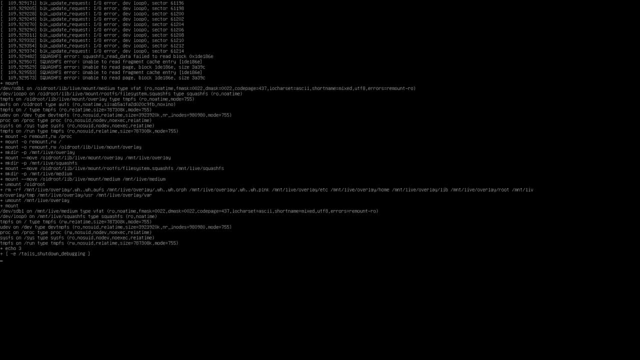 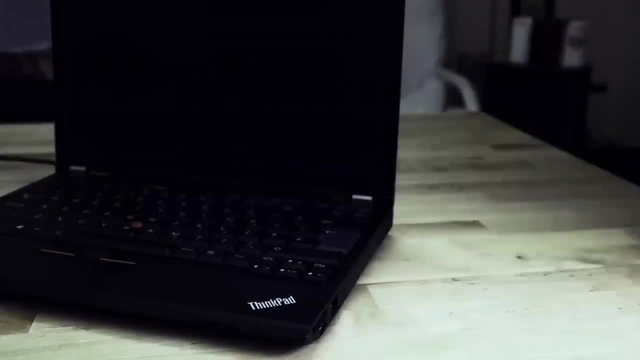 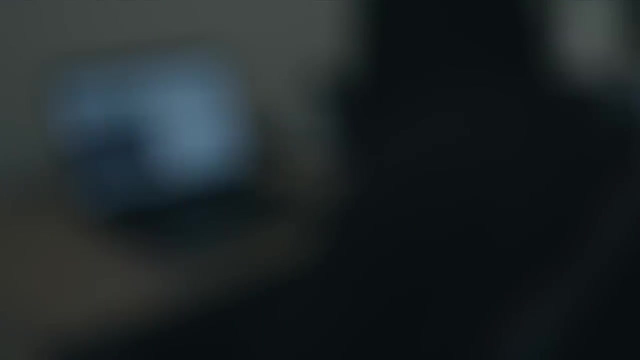 security tool. If you don't have a security tool, you can use the security tool. If you don't have a security tool, you can use the for today. thank you very much for watching and i hope you find this tutorial useful, if you did. 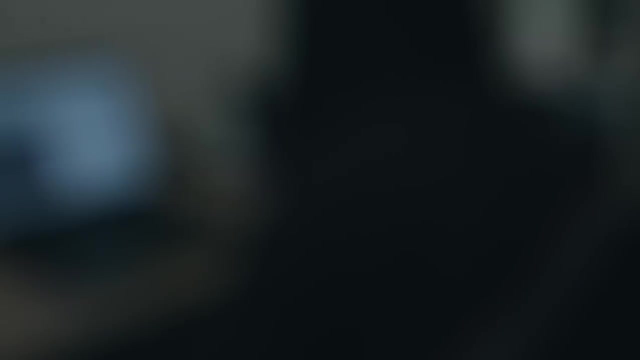 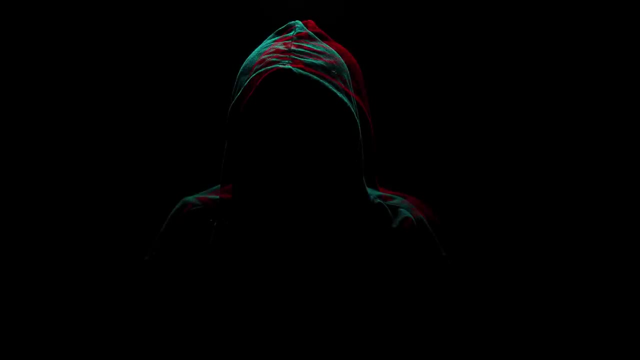 please give it a thumbs up, share this video with your friends and neighbors and comment down below with your questions, or just simply engage for the sake of the almighty algorithm.